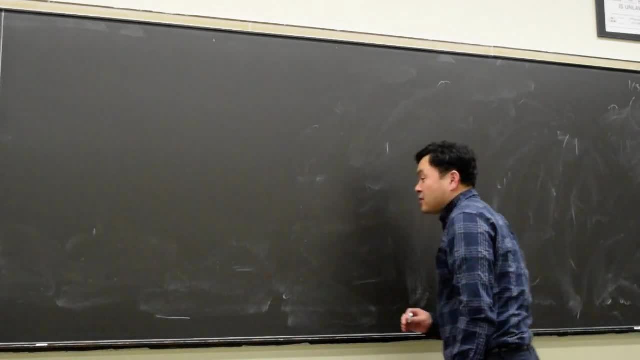 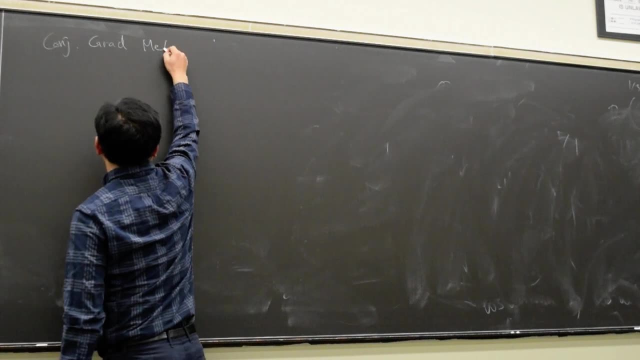 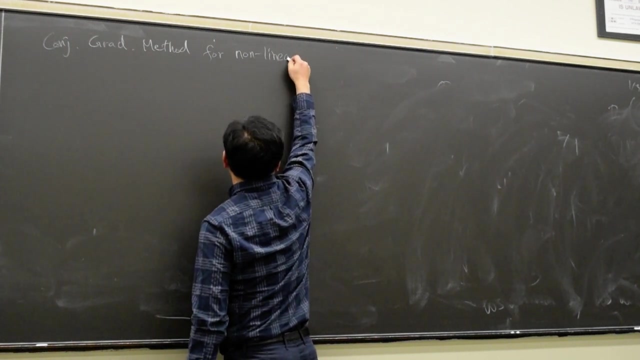 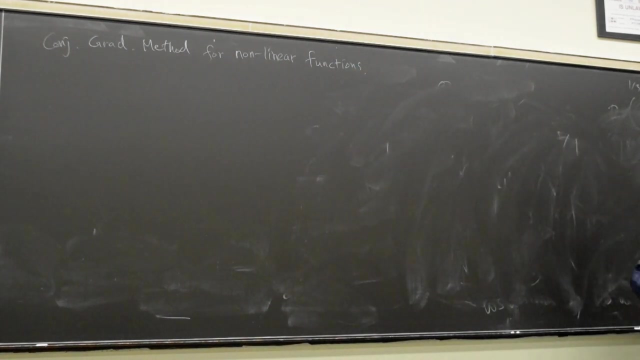 Alright, so let's talk about conjugate gradient methods for nonlinear functions. Now, in order to understand the conjugate gradient method for nonlinear functions, you have to remember what the conjugate gradient method was for the linear function. so let's do a quick review. 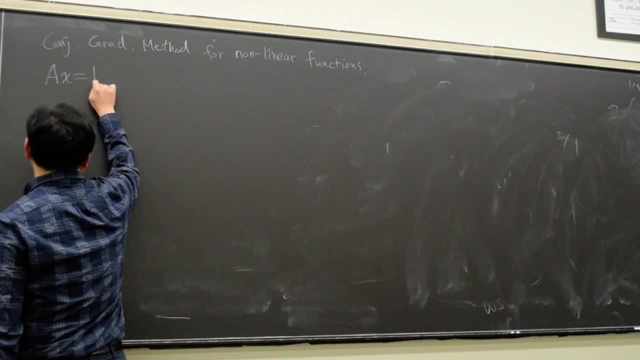 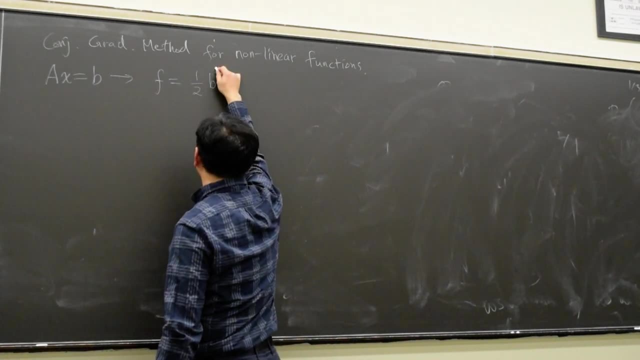 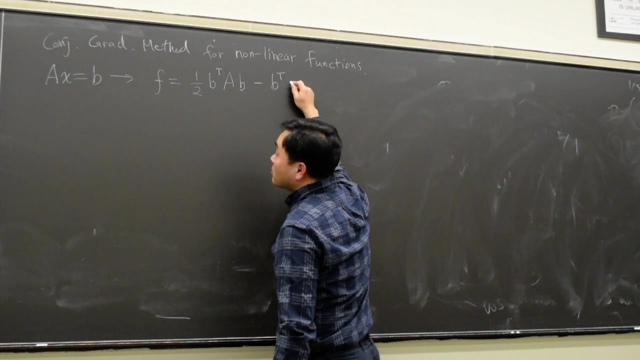 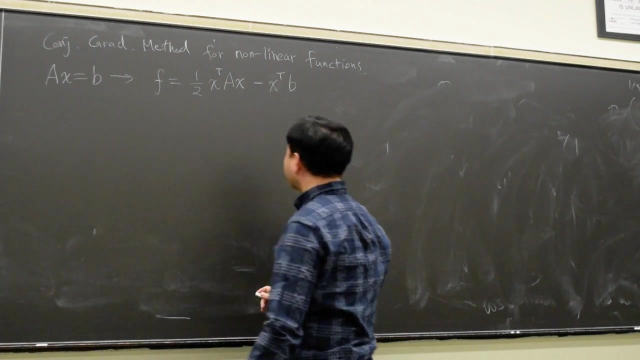 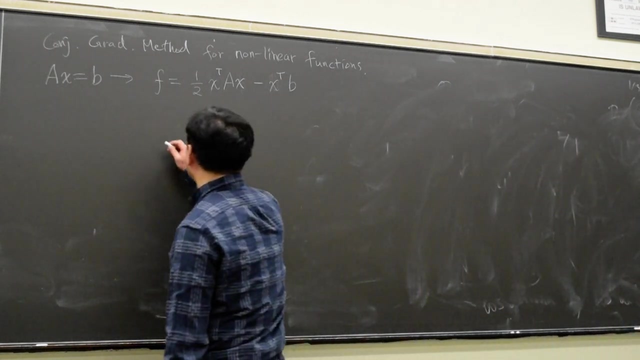 Conjugate gradient method was for solving A is equal to B by minimizing the following functions as one half B, T, A B minus B, T and then actually sorry, this should be X, Then X B. And the reason that this function is good is because, if you calculate its gradients, 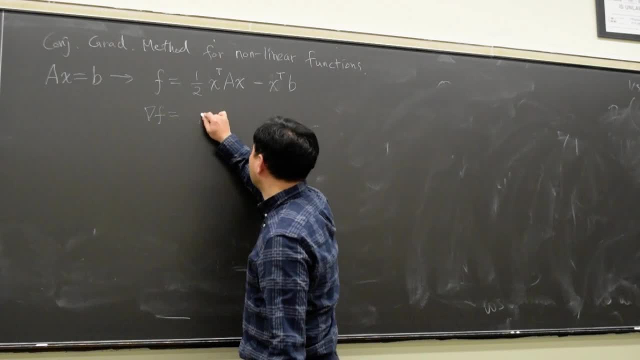 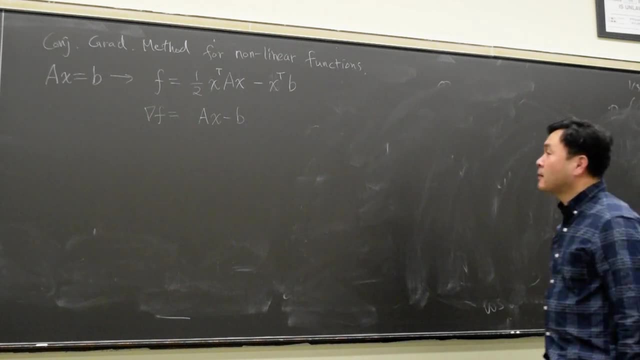 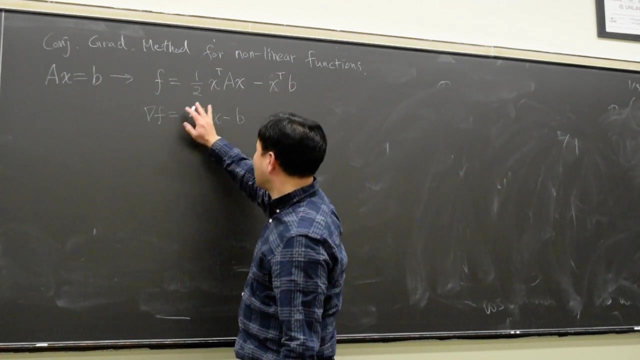 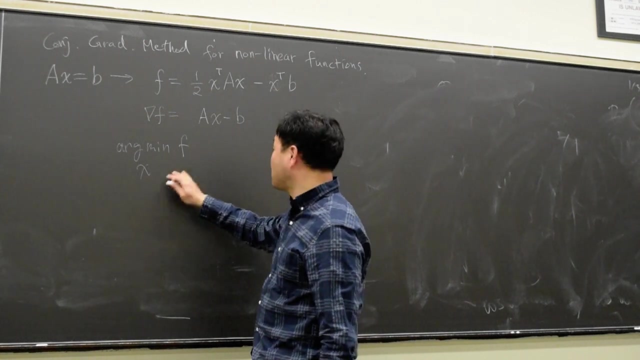 you see that this is. if you calculate it, you're going to see that the gradient just becomes this one, And so when this is minimized, this is going to be zero and therefore the solution- the X value or the vector X that would minimize this- will be actually the solution. 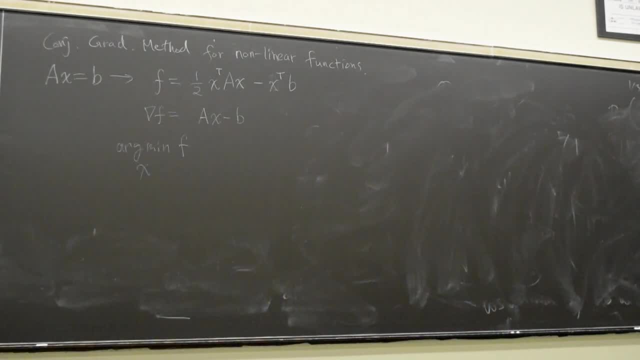 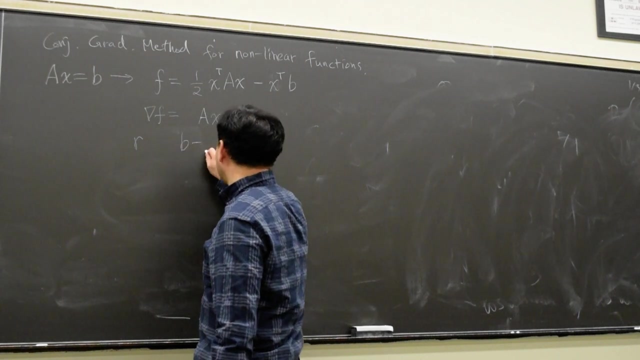 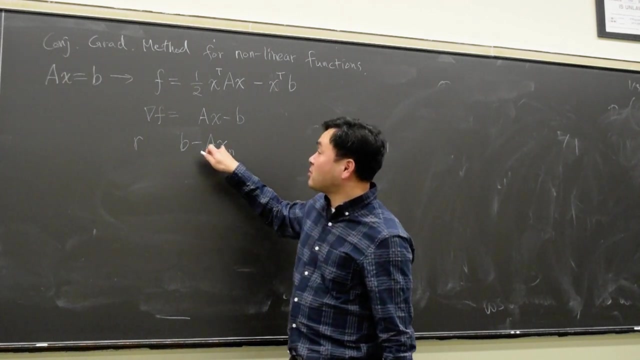 That was our approach And when we were doing this we were doing something like a gradient descent. So see B minus A S. So we're going to do a gradient descent of X for some approximation. So if X, M is an approximate solution of this, 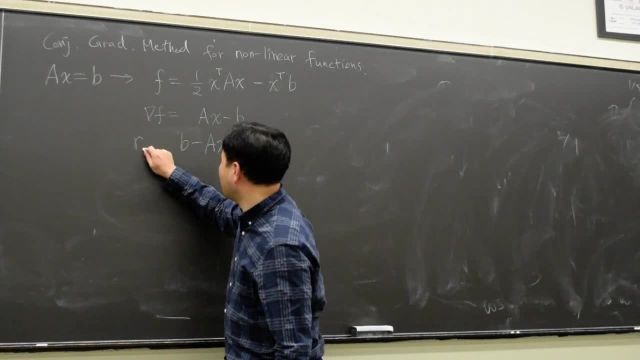 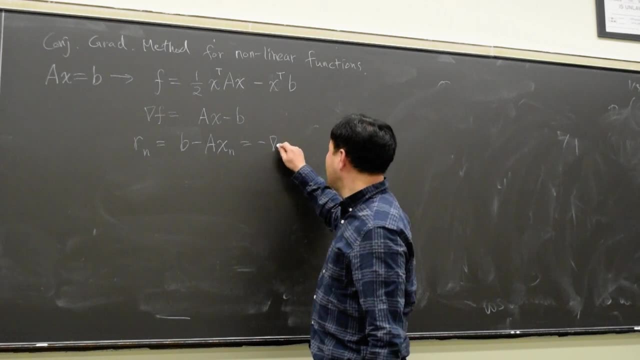 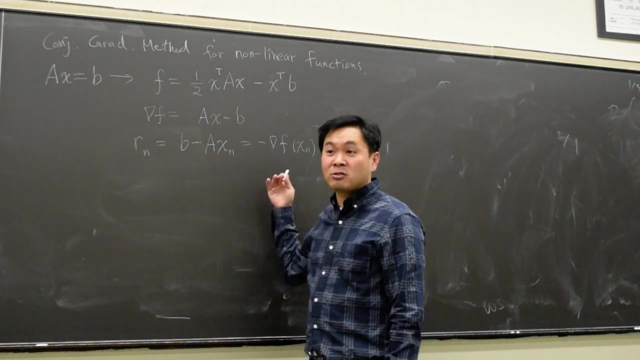 then this is not exactly equal to zero and that's called the residual. And this happens to be actually this with a minus sign. So in this conjugate gradient scheme, always the residual is the direction that you want to. I mean, the residual is the gradient direction you can move. 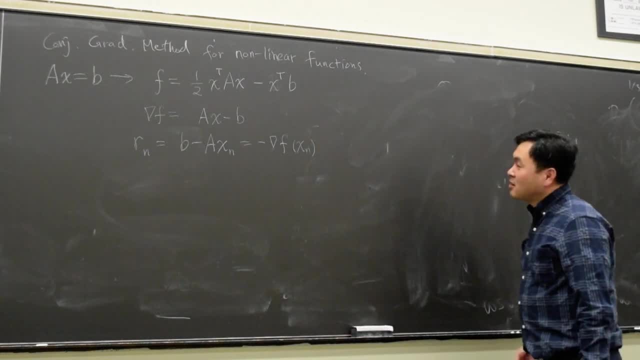 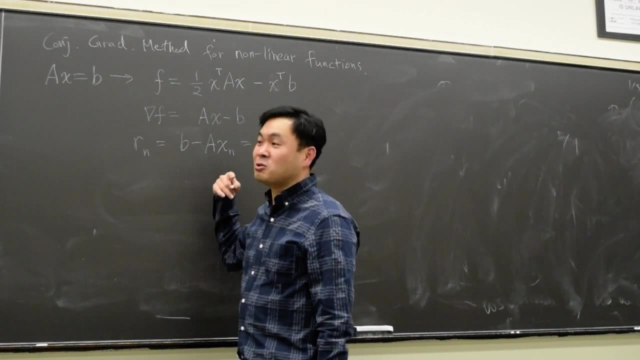 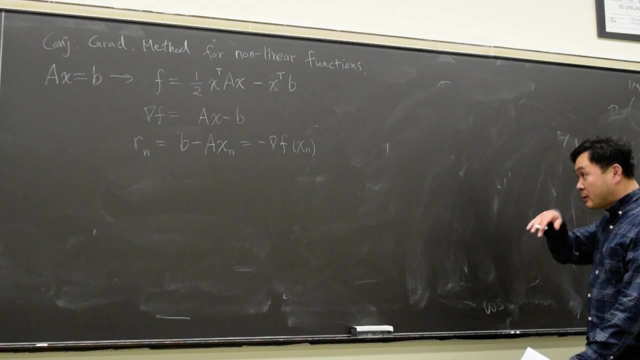 and the conjugate gradient method says: well, you really don't want to move in the gradient direction- negative gradient direction- You want to move in slightly modified direction, which is conjugate direction. So that's where the name comes from. Okay, 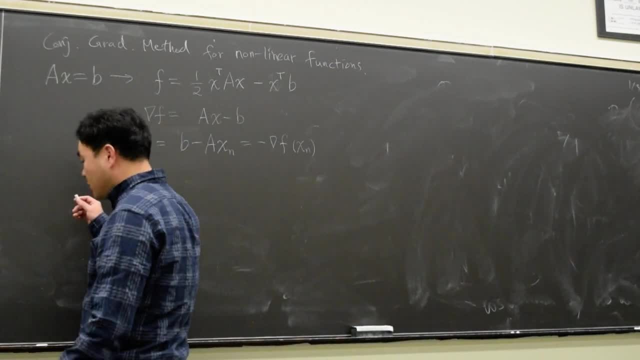 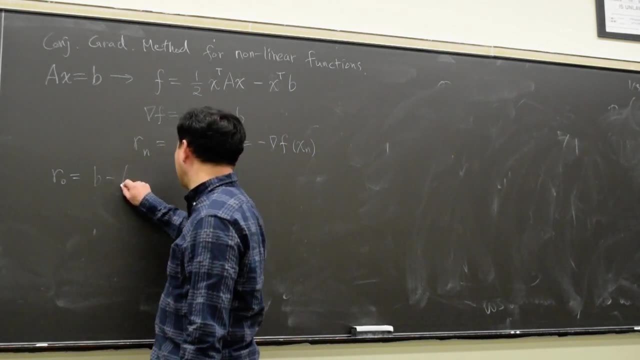 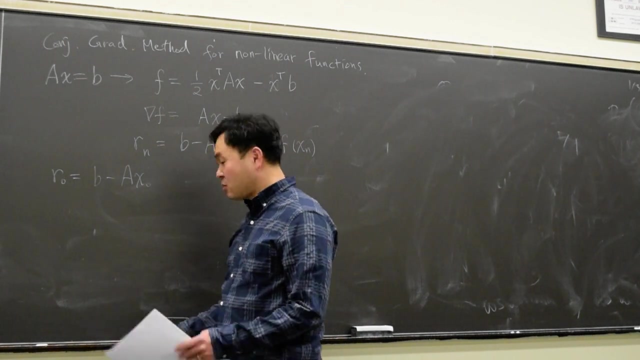 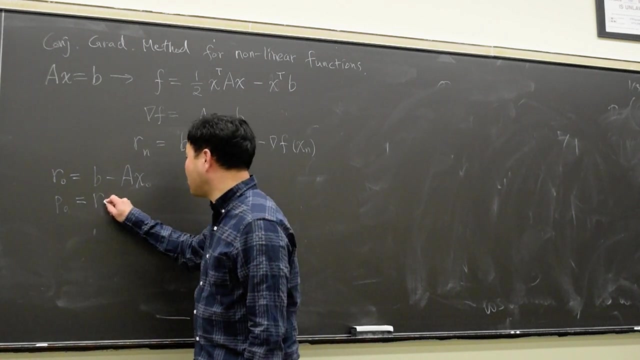 So the algorithm is as follows: First you start with some initial R zero and from some initial point. So this is your initial guess and this is the initial residual. And then in the beginning, your search direction is exactly the same as your equation. 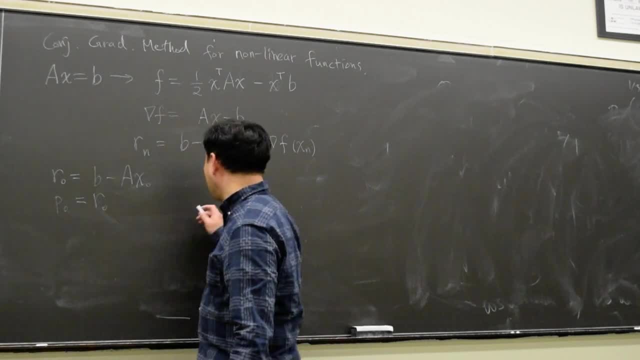 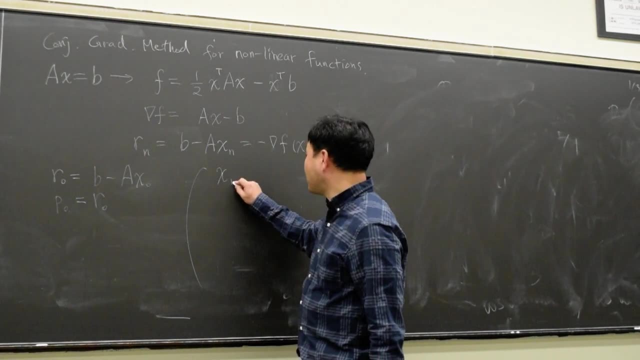 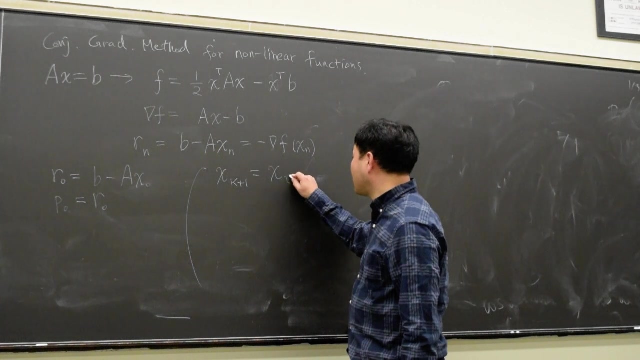 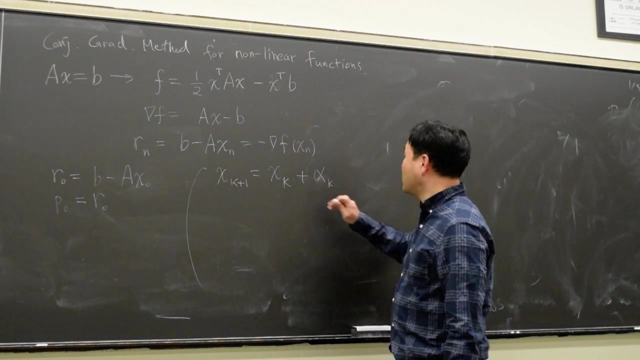 Now, once you have set it up, you're going to do loops, and the loops go like this: Your next spot, your next iteration, the next approximation is your previous approximation. previous approximation plus some number times your search direction. Okay, 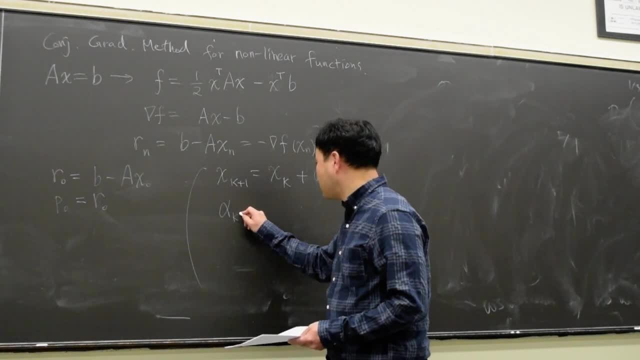 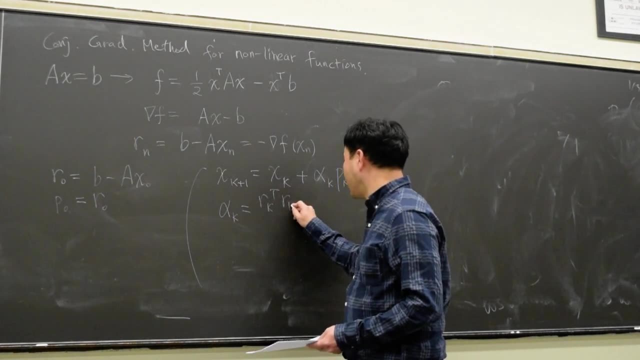 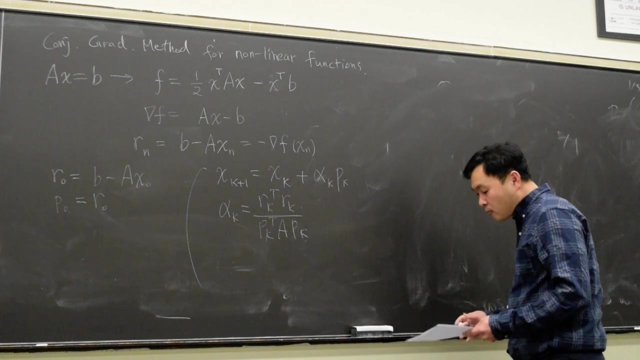 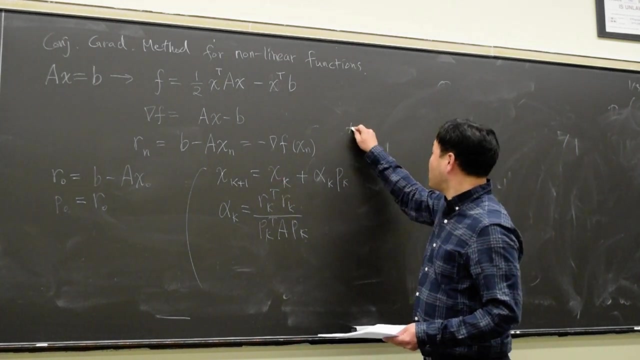 And we prove that this search direction is optimal if alpha key is r k, t, r, k, over p k, t, a, p k, And this is so in this line. so, starting from this point, x, k, if this is p? k search direction, 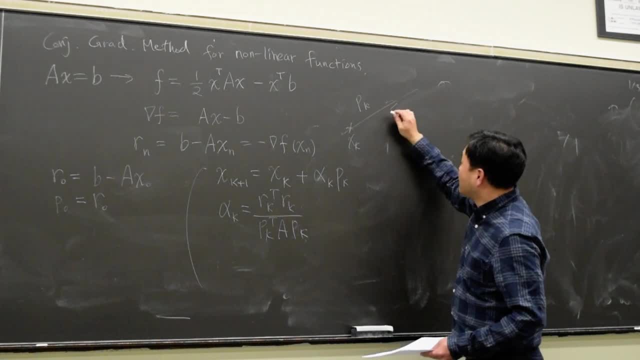 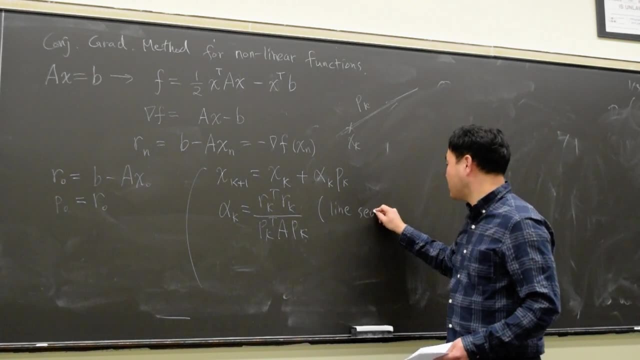 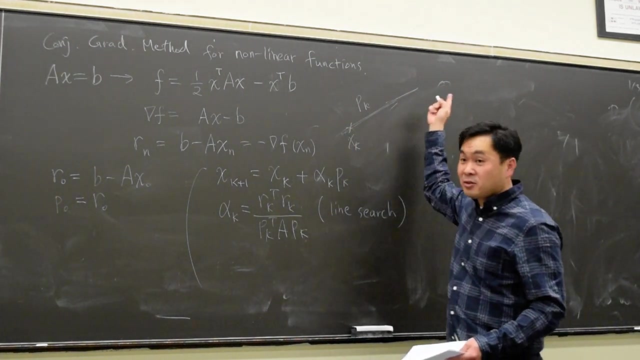 the amount that you have to go is exactly this much. So you're doing a line search. This is what we think. We're doing a line search, And this gives you the minimal value of this function on this line. So you're doing the best possible movement at each step. 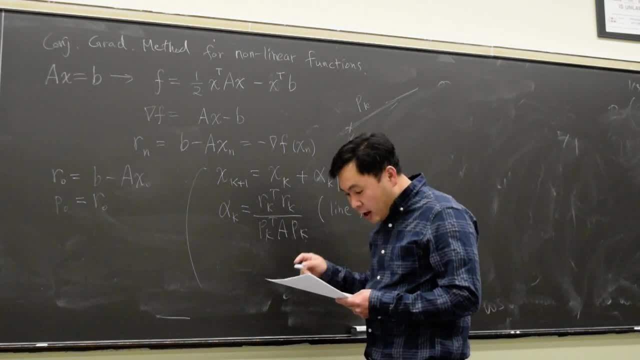 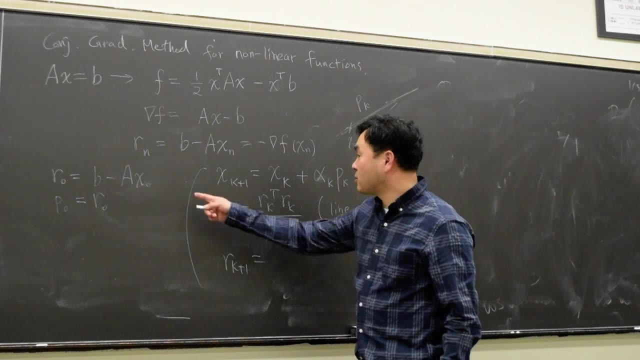 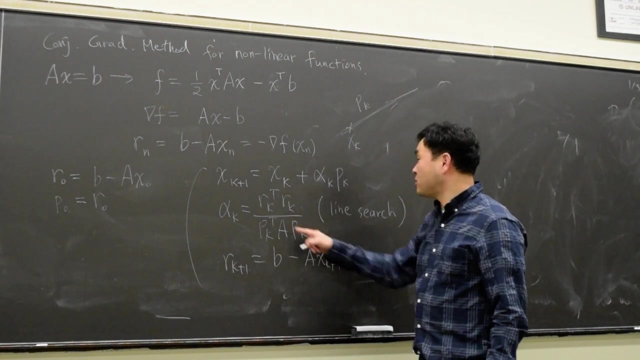 Okay, And then, after this you define, you can calculate the next. you can calculate the next difference. So b minus. since you have a new x k plus one, now you can use this x k plus one and calculate its residue. 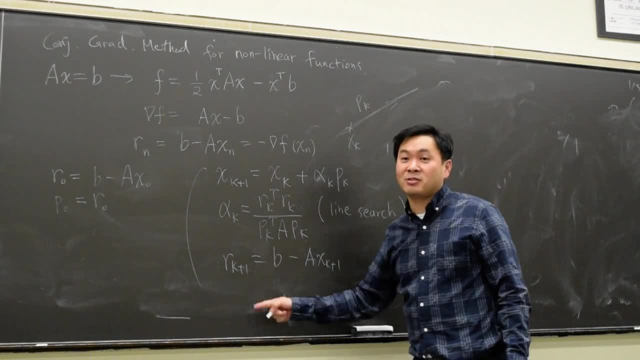 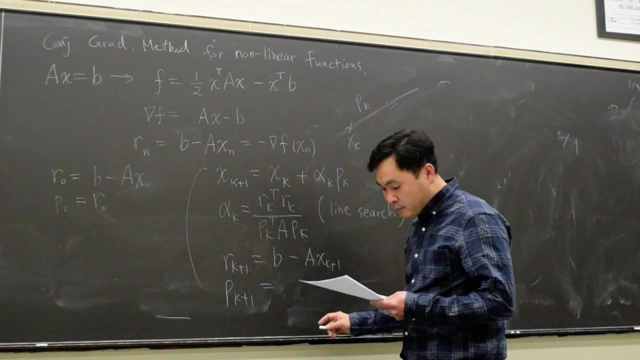 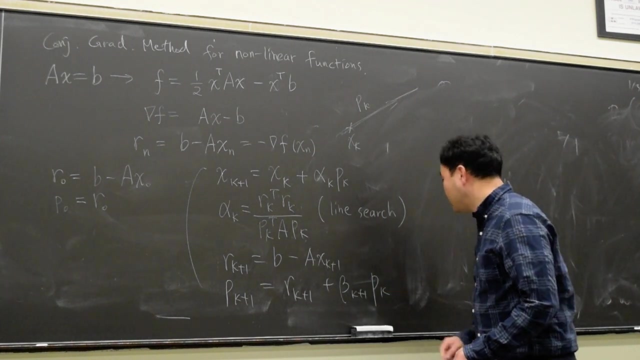 That will be your new gradient direction, but you're going to modify this to a conjugate direction And the conjugate direction is p k plus one, is r k plus one plus beta k plus one times p k. Where this beta k plus one? 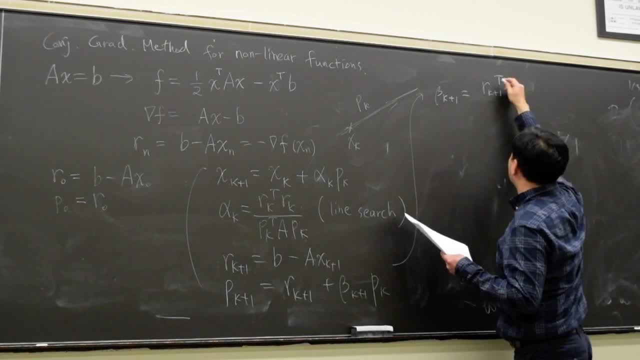 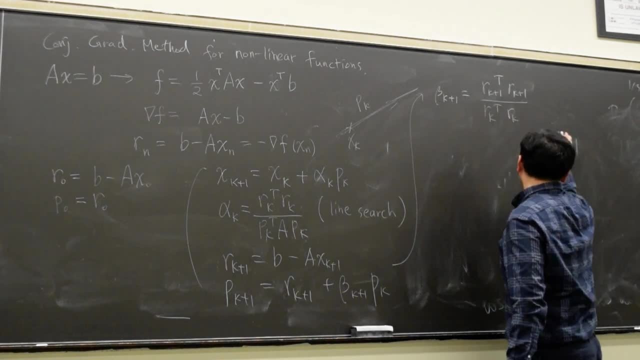 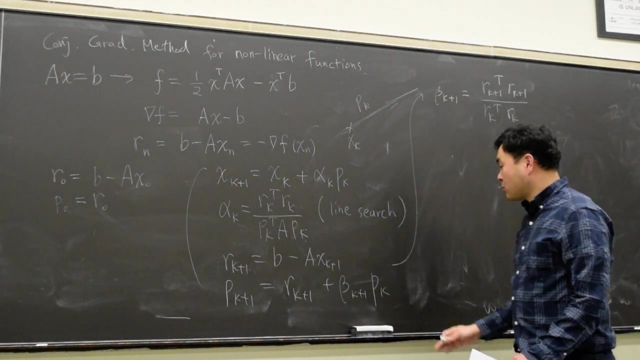 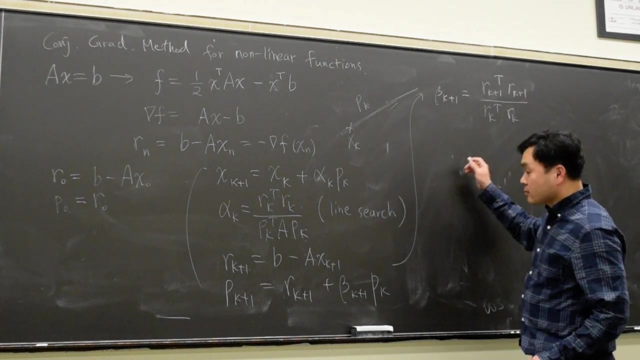 was obtained at r k plus one, transpose r k plus one, and r k transpose r k. Okay, And this conjugate direction. this has to be done, this has to be calculated so that your, your p k plus one and p k's. 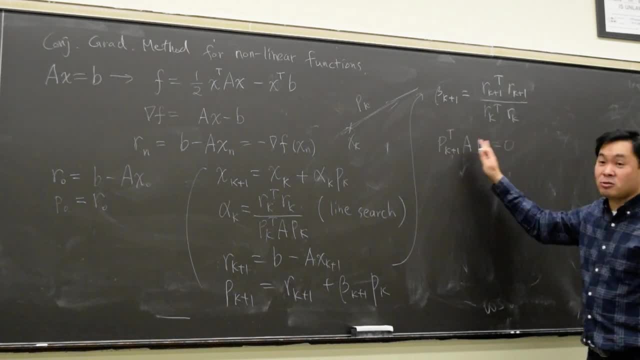 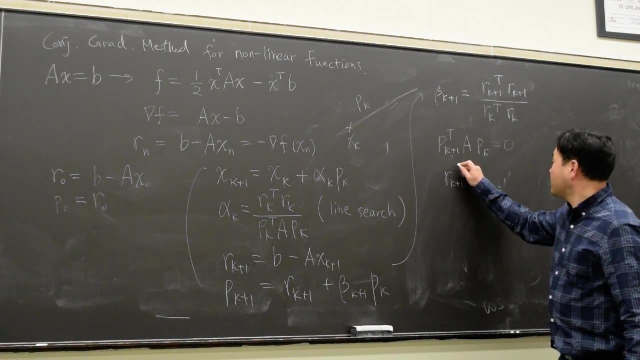 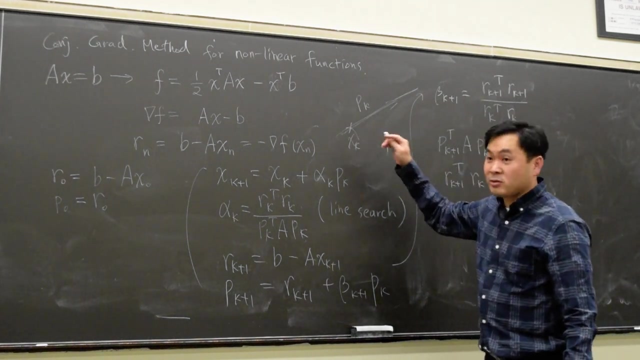 are conjugates. Okay, So being conjugate to each other means it's orthogonal. with respect to this norm And the residuals themselves, you can show that these are always, always, at each point, the residuals will be orthogonal to each other, So the gradients are orthogonal to each other. 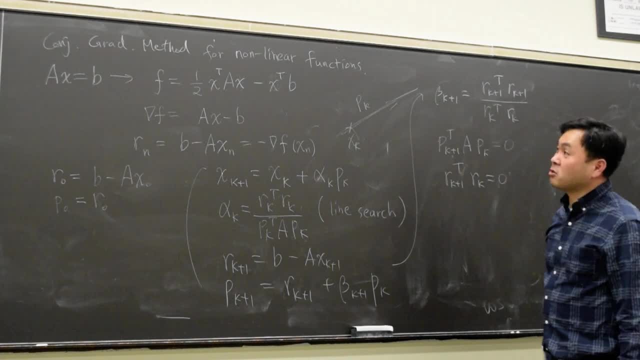 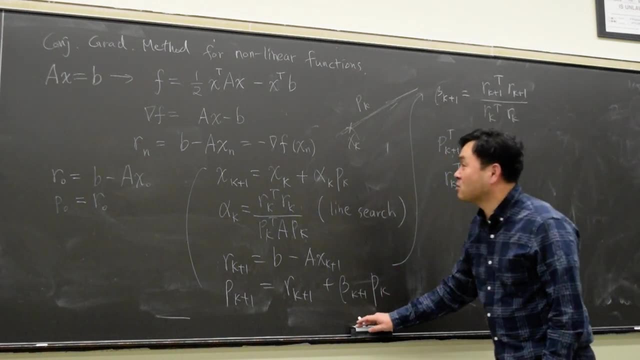 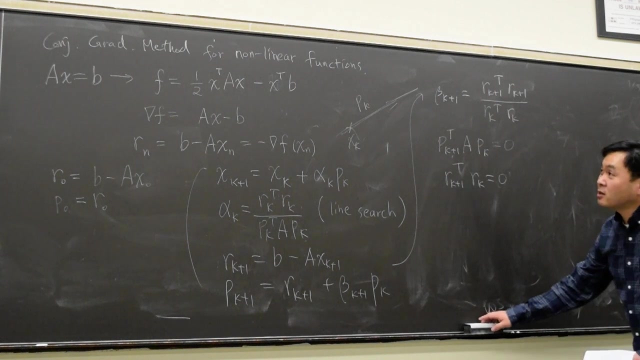 Search directions are conjugate to each other. So that's the conjugate gradient method, which I recorded in the previous video, and you can review it if you need to. Okay, So now what is the conjugate gradient method for nonlinear functions? Well, 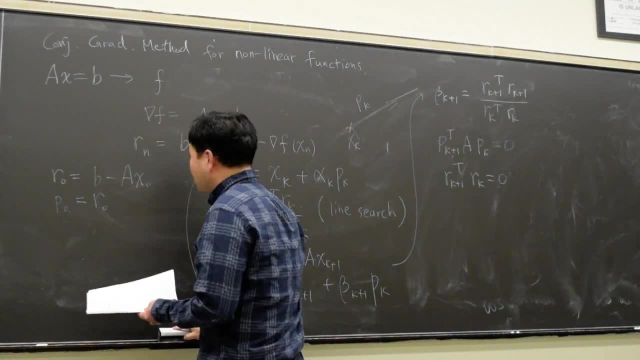 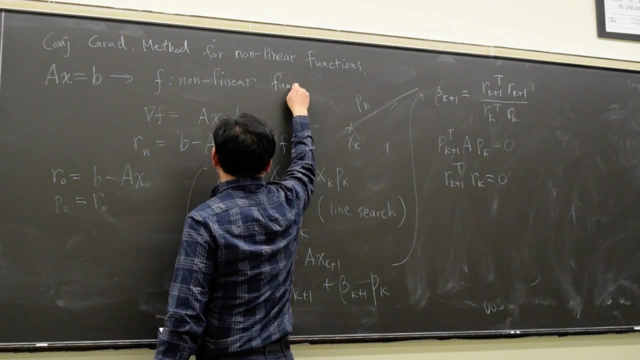 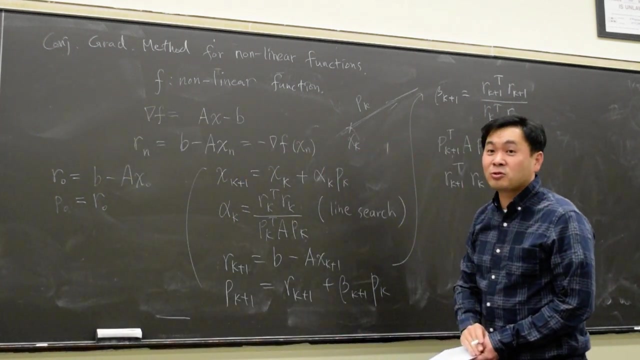 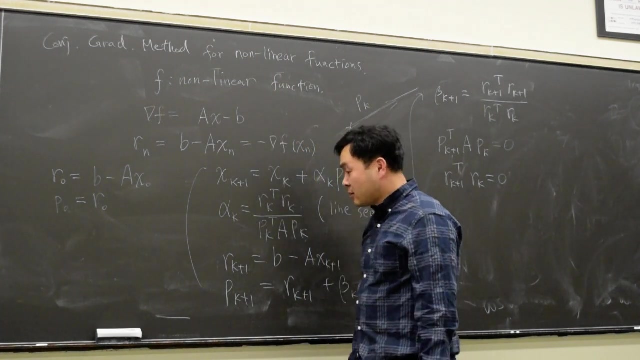 you assume that your function is just some nonlinear function And your goal is not solving a linear equation anymore. Your goal is just to find the maximum or minimum, actually find the minimum of this function. Okay, To find the minimum of this function. 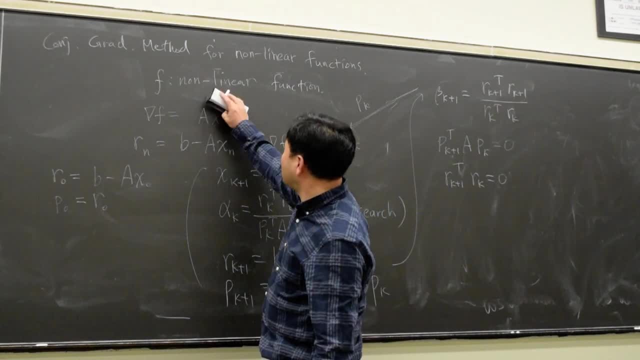 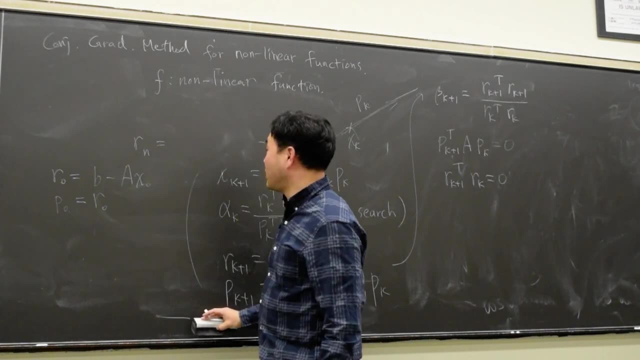 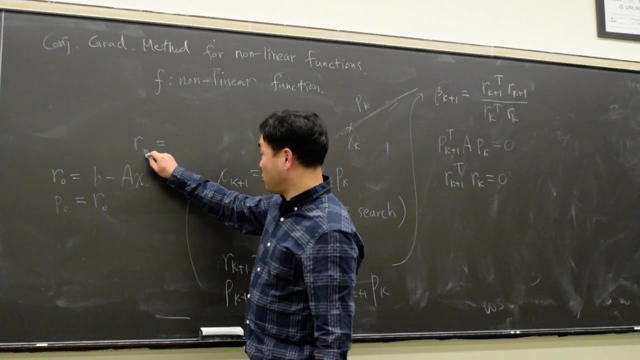 what should we do? Well then this: this is no longer true, But what we can say is that, instead of using the residual, we can say that the gradient direction should be called Rm, So what we call the residual will be just the gradient direction. 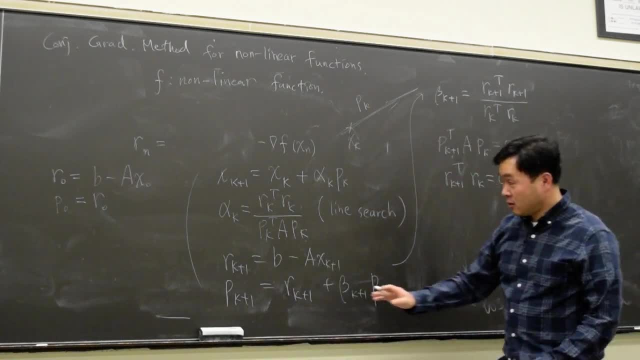 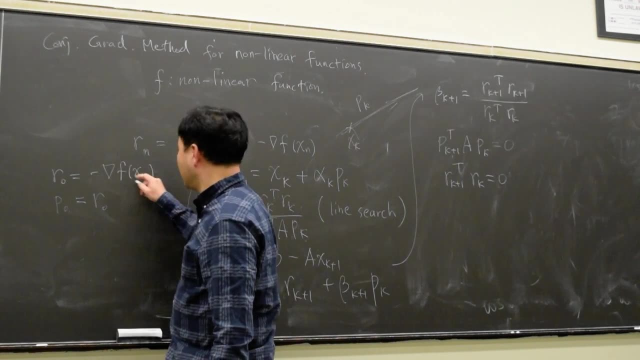 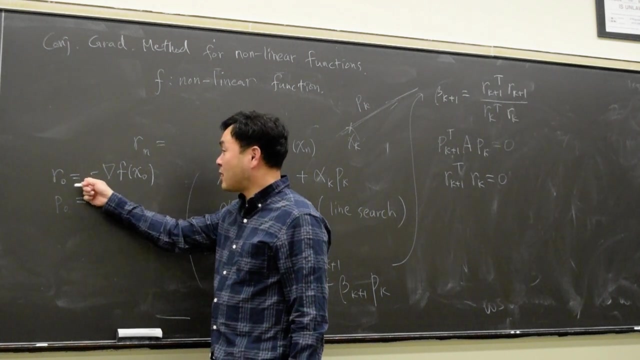 negative gradient direction And this so therefore, initially we'll be calculating this. So calculate the gradient at a given guess starting point and put a minus sign. That will be your R0.. And P0, initially will be the same as the R0. 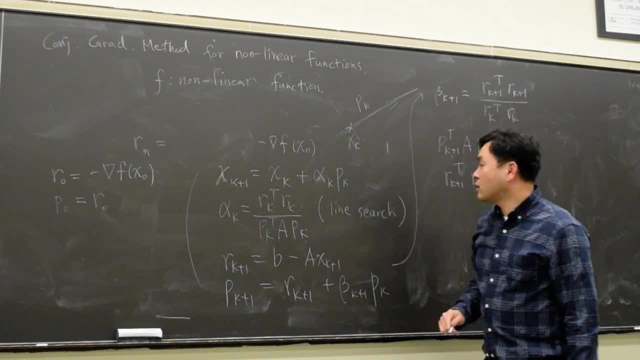 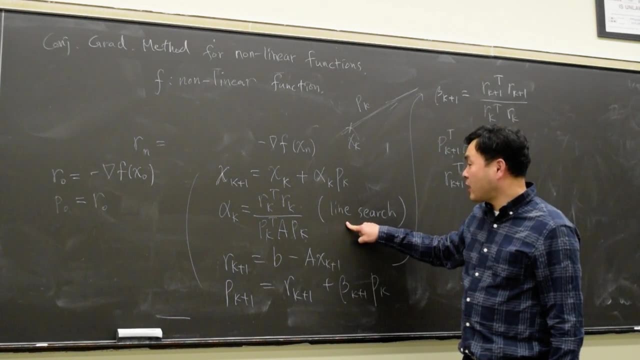 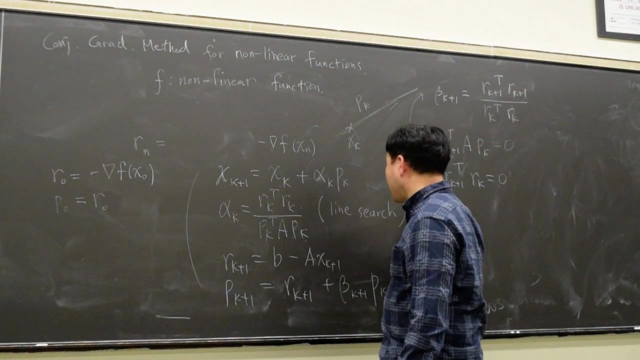 And then you again do a line search. Okay, And if you think about the line search, this doesn't make sense anymore because we don't have the matrix A. So instead of saying that we're doing this, we're just going to say that. 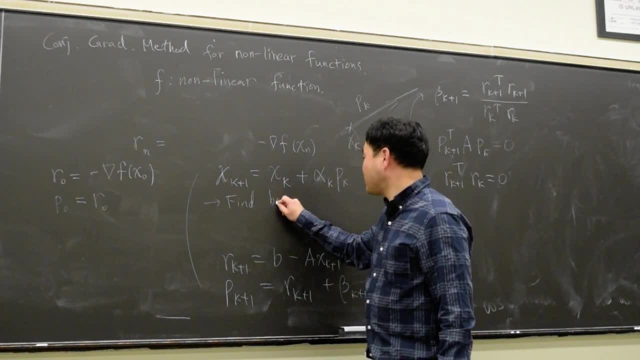 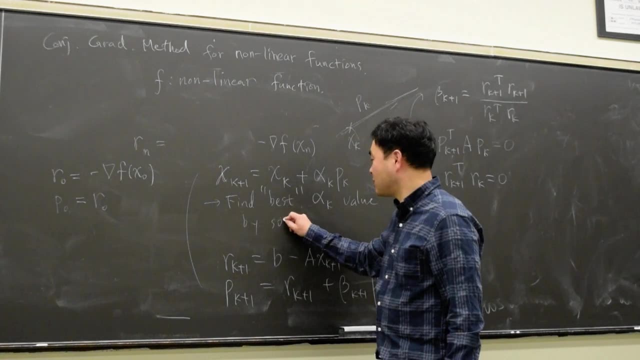 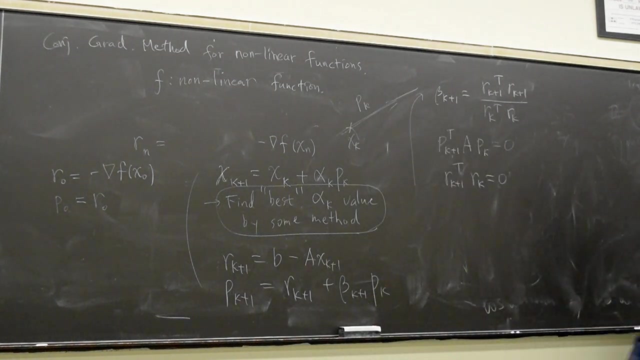 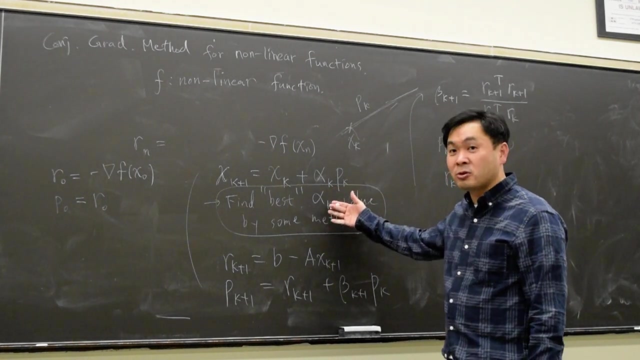 here find best alpha k value by some method, And this is actually the main difference between the linear conjugate gradient method and the non-linear one. I'm going to explain to you two methods that people use in order to get this. And then 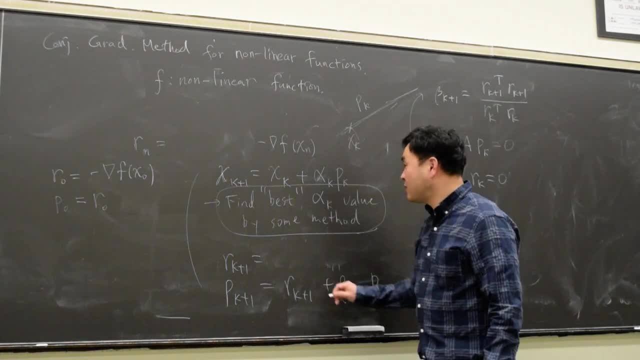 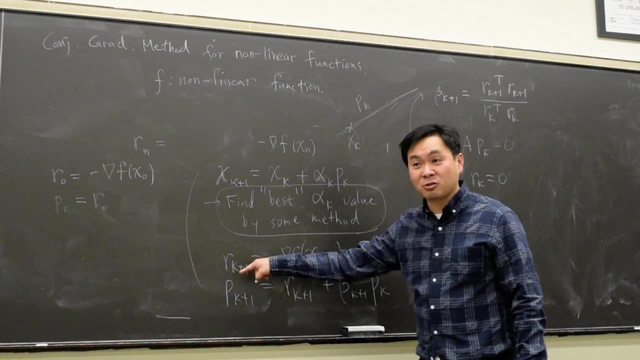 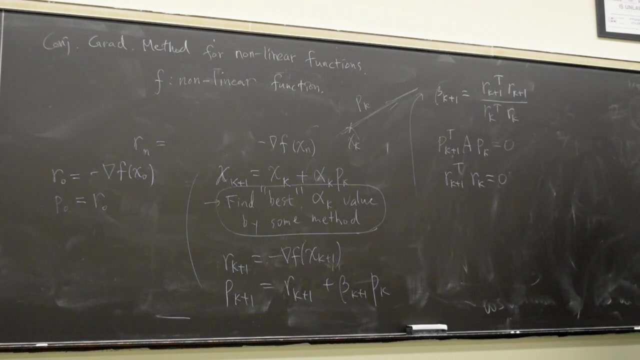 of course this is not true anymore With that new given approximation. you calculate its gradient. for the minus, that's your Rk plus one, And then you have this: And for the beta, k plus one. here there's no matrix A. 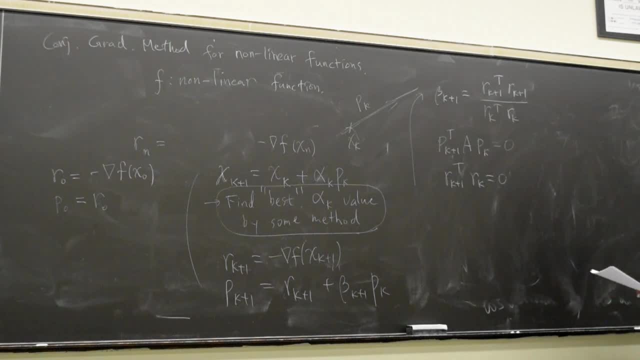 So this still makes sense. It still makes sense, so you can use it. However, it turns out that that's not the best one, So you could use this and using this as your beta k plus one is called the Fletcher-Reeves method. 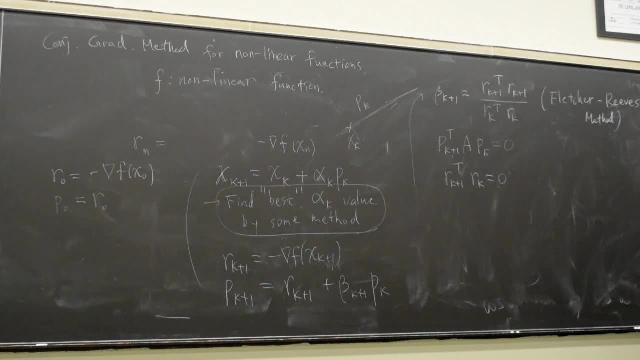 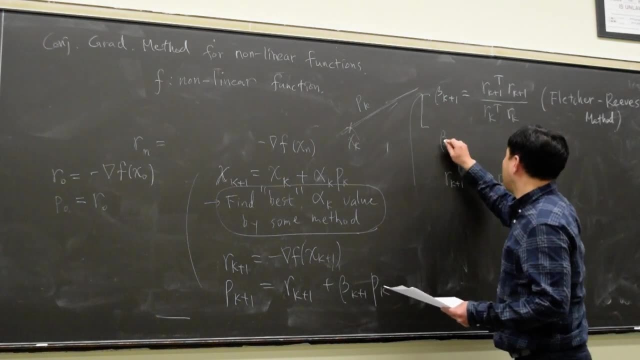 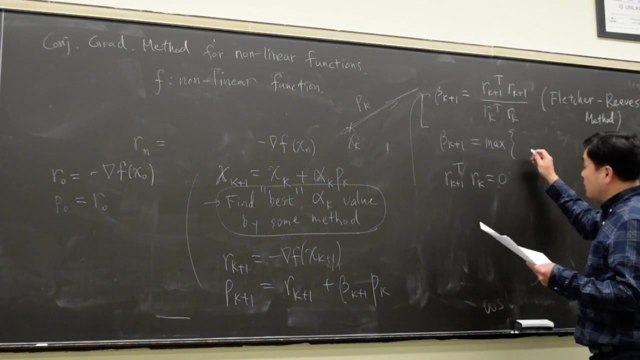 But for some reason. for some reason, the following one is better. So instead of this you can use beta k plus one equal to the maximum of Rk, plus one minus Rk over Rk. transpose Rk and zero Now. 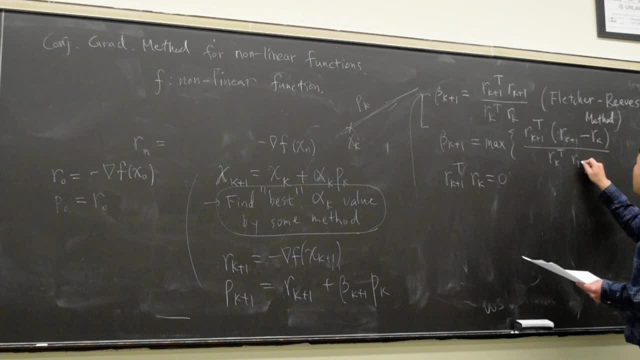 in other words, if this value gives you positive, then use that. If it gives you negative, just put it at zero. So in that case the search direction will be exactly the same as the gradient direction. Okay, And then? 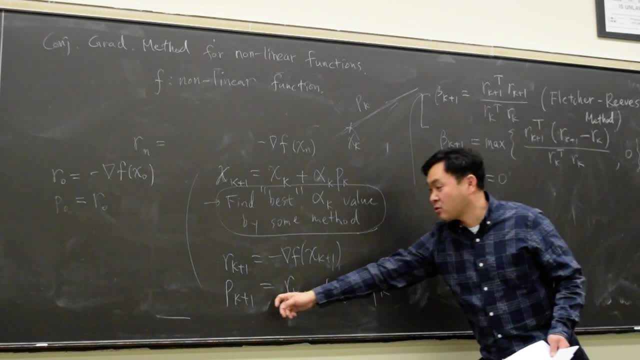 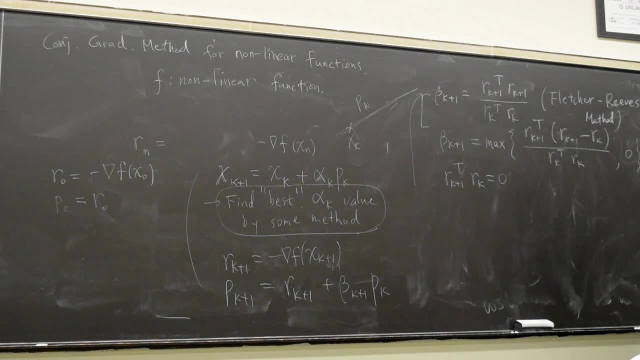 you can use this as your beta: k plus one minus Rk. over Rk transpose Rk and zero. Now, in other words, if this value gives you positive, then, if you look at this, well, this was only true for the linear case. 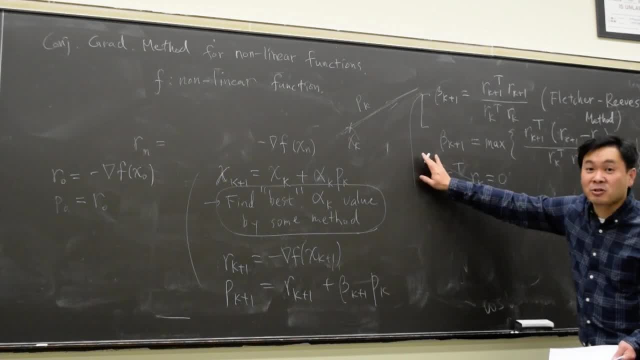 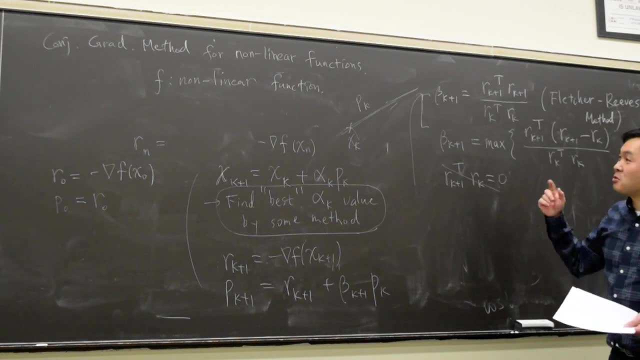 This is no longer true. Okay, Neither is the other one, the conjugate direction, true. So, when it comes to nonlinearity, saying that the search directions are conjugate to each other somehow doesn't make sense, but it kind of makes sense. 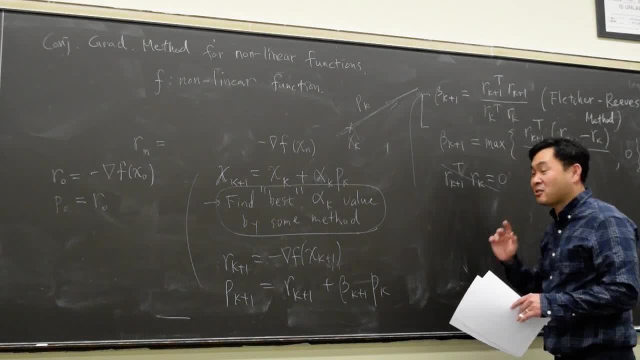 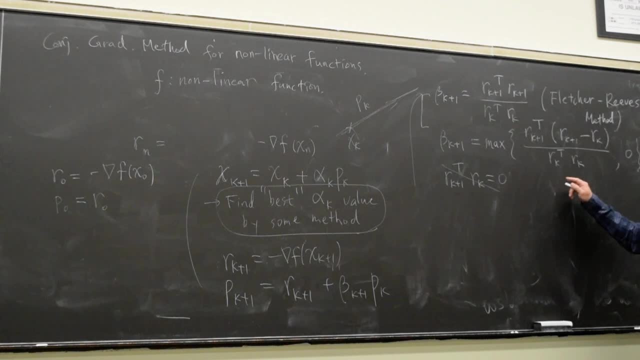 You can make sense out of it a little later. Let me explain that a little later. Okay, So this is not true, but what I want you to see is that in the case of the linear, this dotted with this one would be zero. 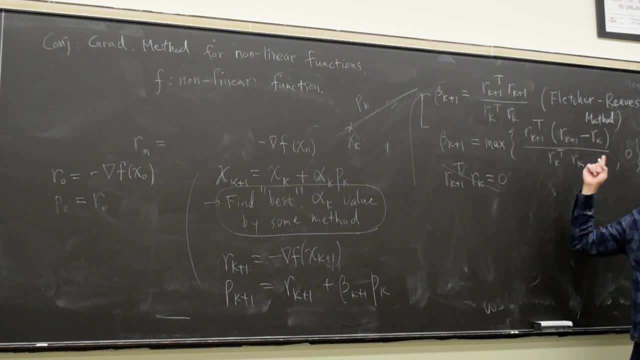 Right, So for the linear case, this and that are the same thing. It's nothing different. Okay, So it's. oh, and by the way, using this is called the. what is this called? I forgot to write it down. 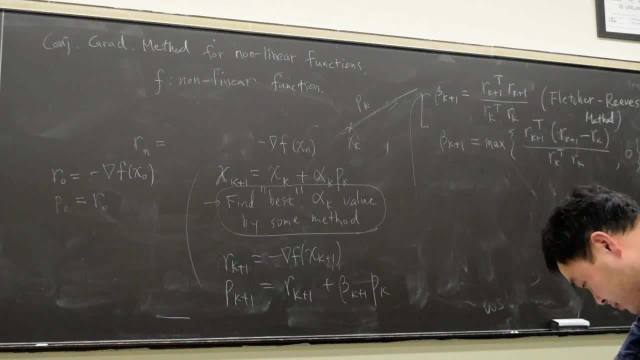 Let me look here. It's Pollock-Riviere, So this is called Pollock-Riviere Magnet. Okay, So there are these two common choices and there are a few more that other people use. If you think about what this is doing, 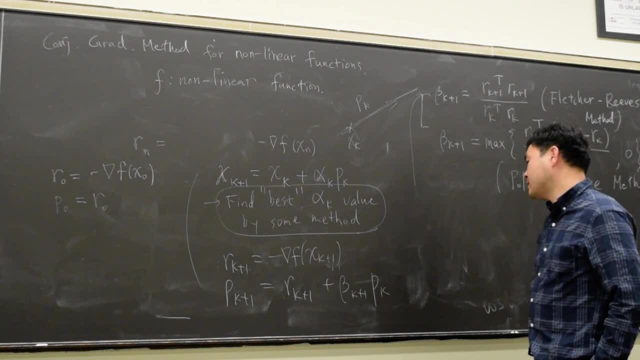 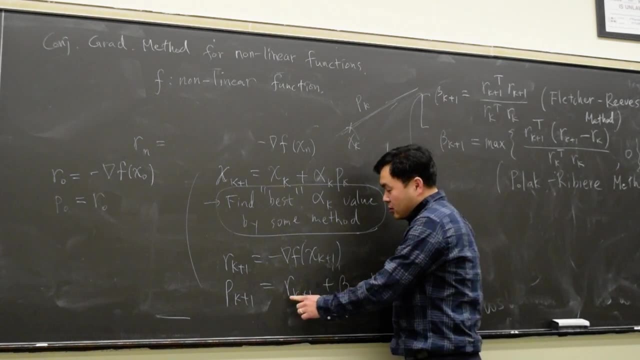 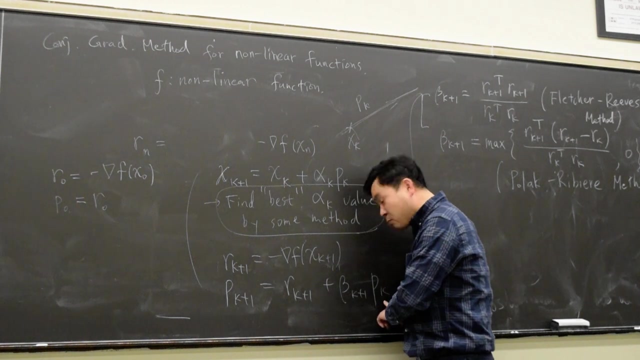 it has the following flavor: See to say that you have something positive here is like you're trying to move at the gradient direction, but you're modifying it. you're remembering your previous search direction and adding it and going a little bit towards there. 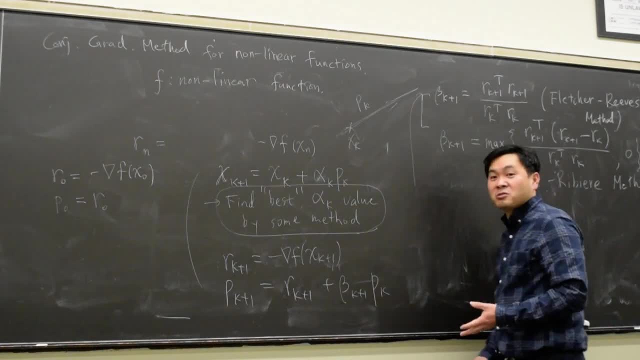 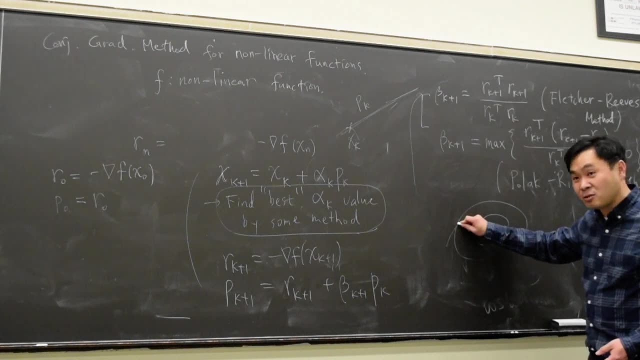 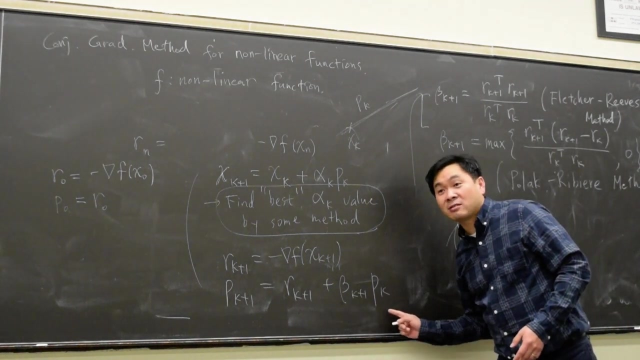 Okay, And actually people who do machine learning realize that often when you try to minimize a function and you do gradient descent, your gradient descent, like, goes zigzag and takes a long time to get there. And if you use this, 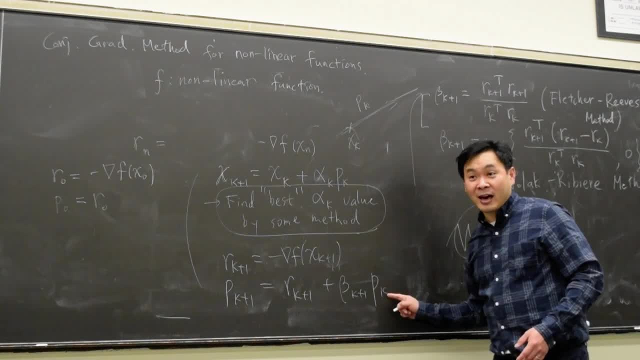 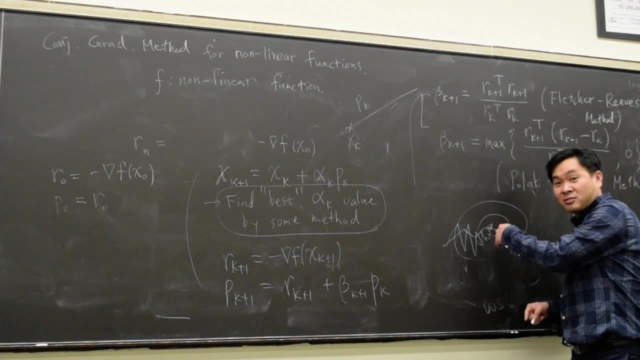 what they call this momentum. if you use your previous values and add it, add that in that case this actually is less wiggly and it converges to the minimum gradient. So I don't know if they knew the conjugate gradient. 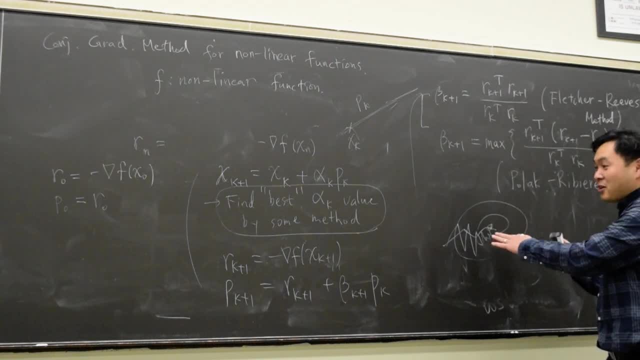 method for nonlinear functions. but at the end of the day they kind of figured out that that's what you have to do. So people who are doing machine learning actually is doing this without maybe they know. I don't know They're doing this. 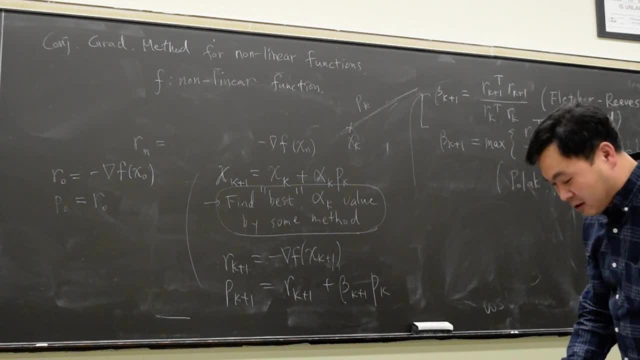 Okay, All right. So now, as you can see, there's not much of a difference between the original one and the nonlinear one, except for the case of this part. We just have to explain what to do at this part and we can say: 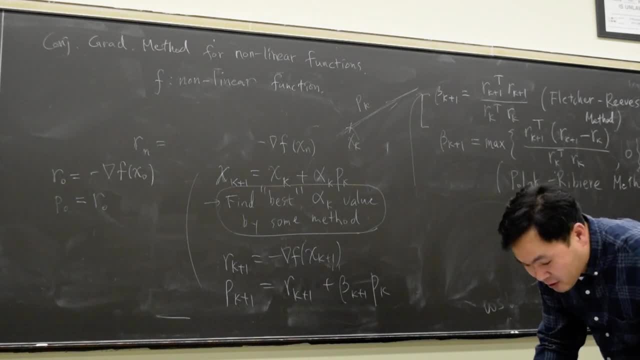 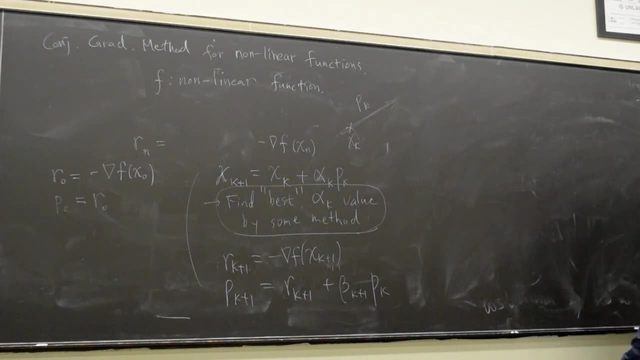 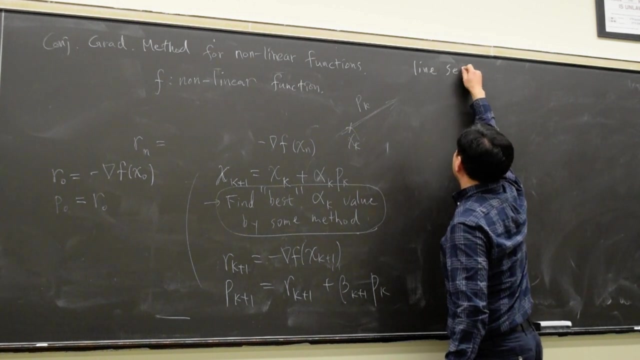 that we've covered this. So let's see, There are two methods in dealing with this. What does it mean to be choosing the best possible? Well, first so the line search methods. there are two. One is Newton-Raphson. 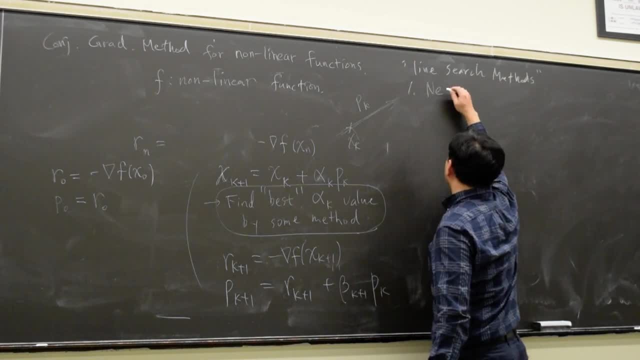 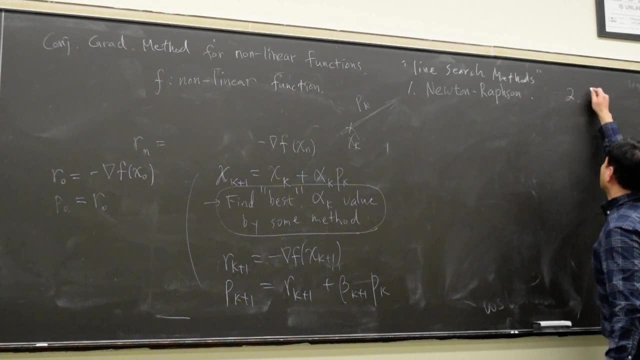 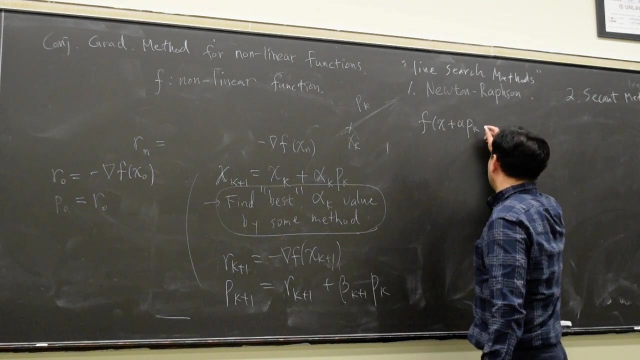 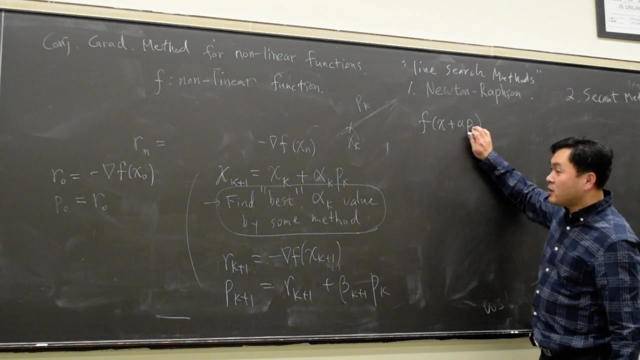 Newton-Raphson. And the second one is sequence method. And let me explain the Newton-Raphson. first, You use the Taylor series. you use the Taylor series and you use the Taylor series of this search. So let's say your p. 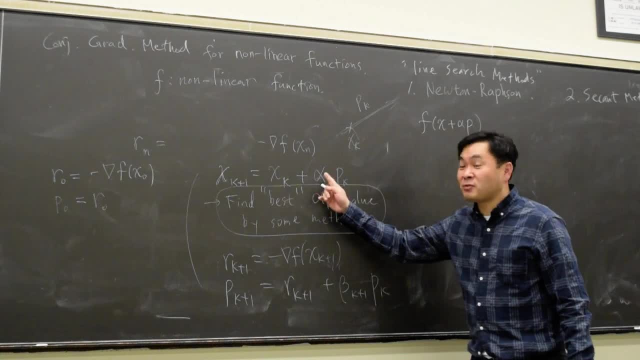 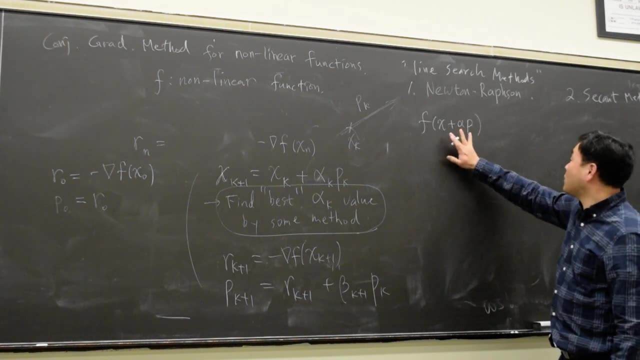 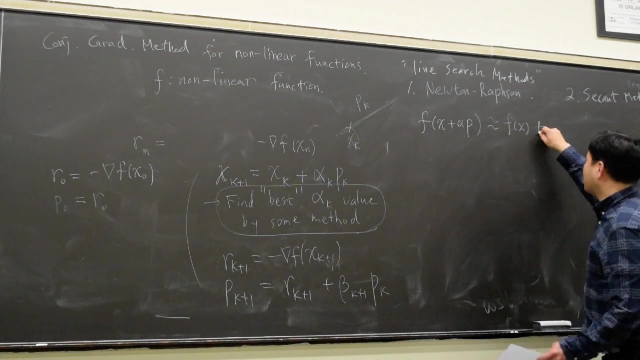 is. you figured out your p, You know which direction you have to go. You just have to figure out how much you have to go. So you have your initial beginning point and you're trying to figure this out. So you have. 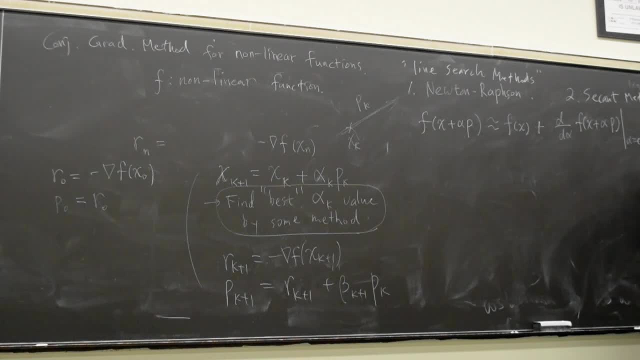 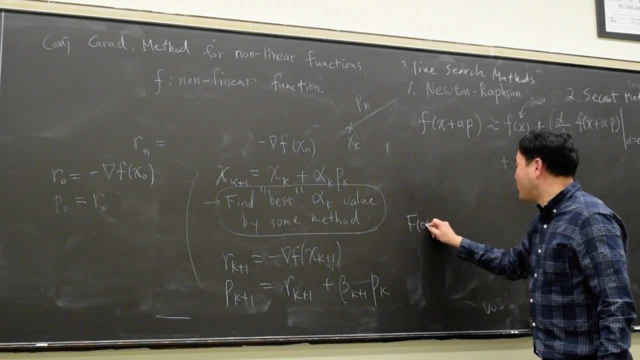 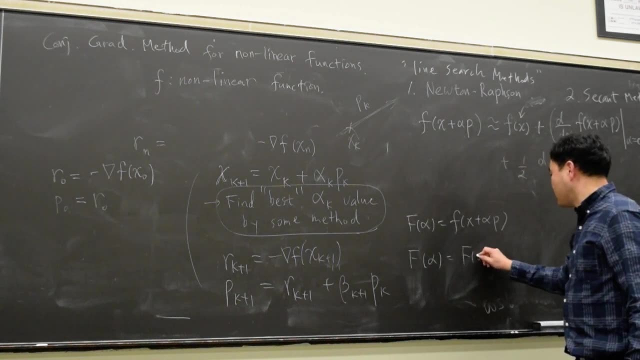 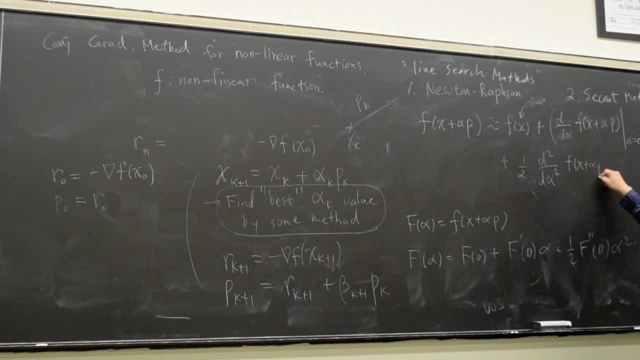 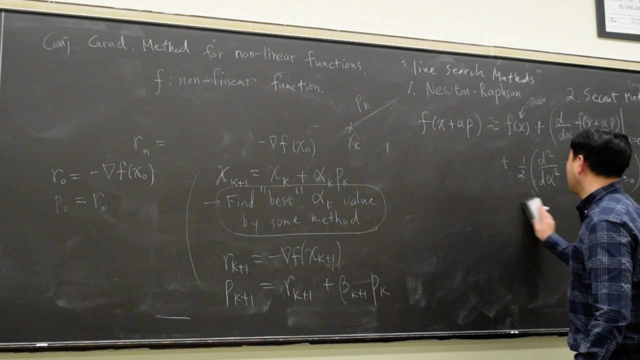 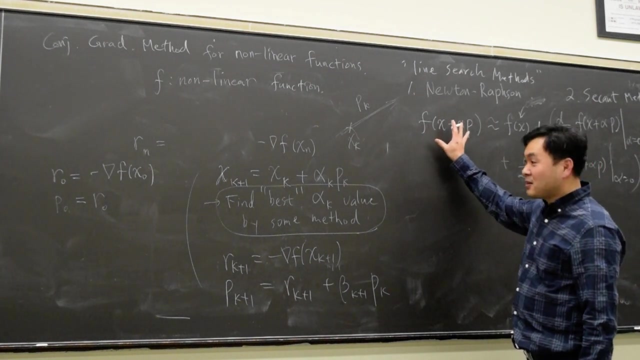 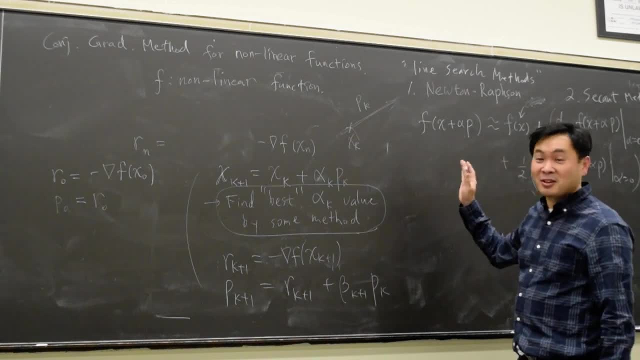 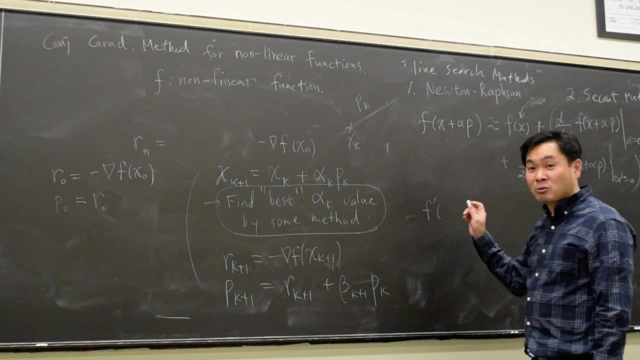 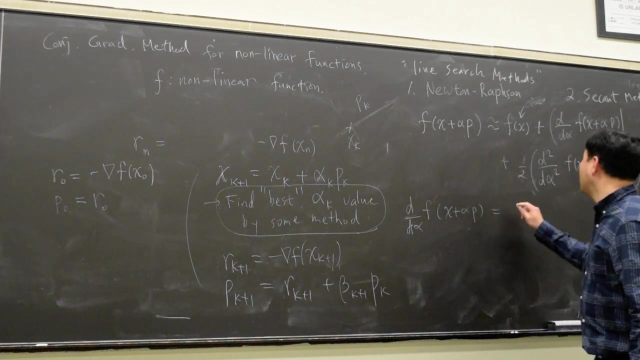 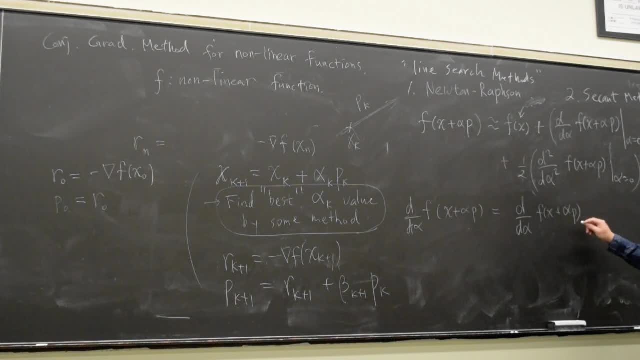 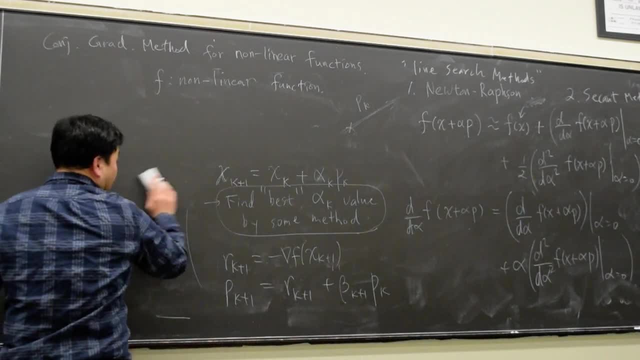 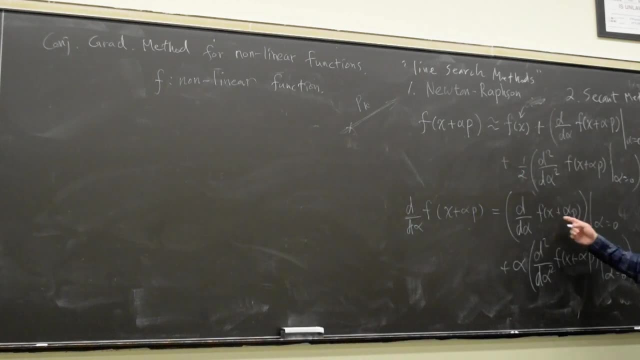 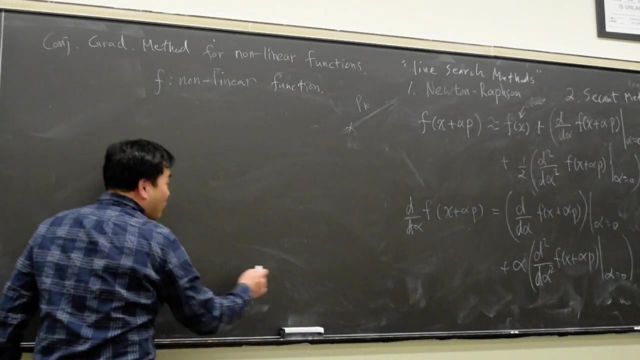 Okay, now look, You have a function, multivariable function, and you're trying to find its change along one direction. That's directional derivative, right? So you can rewrite that as: so I want this to be zero, So I want it to be like this: 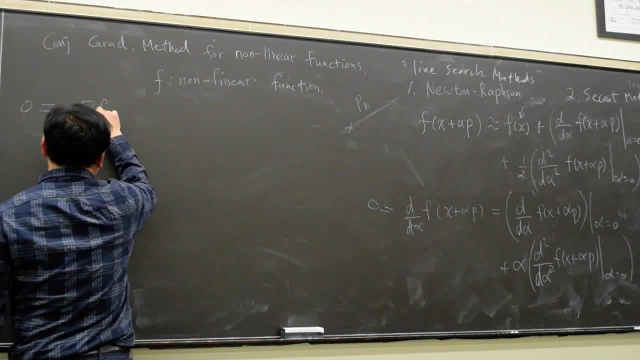 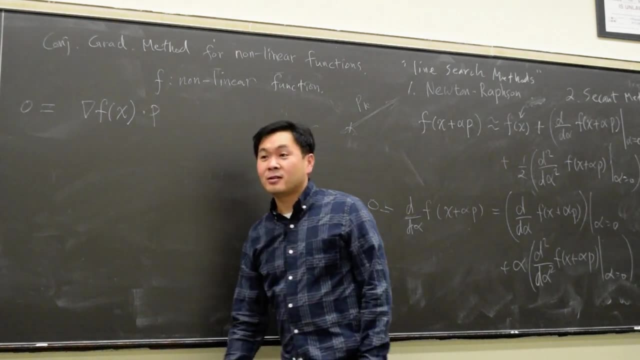 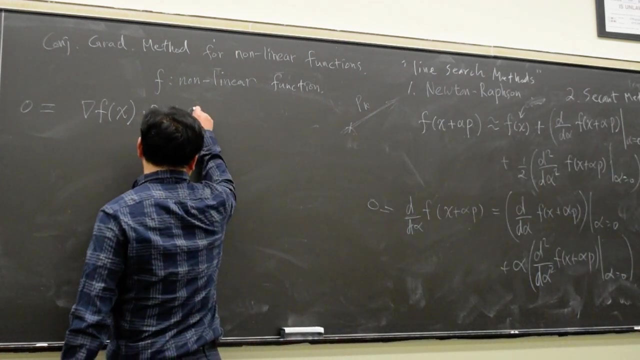 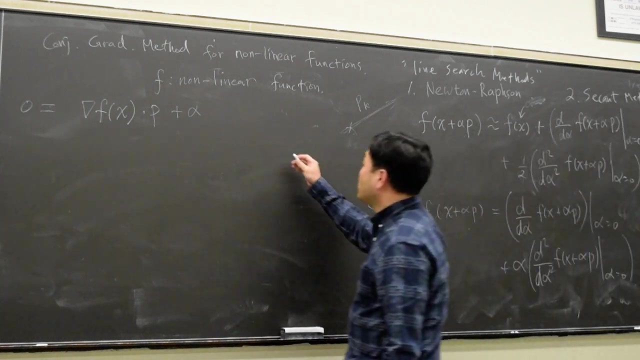 zero equal to gradient of f evaluated at x times dotted with p. So that gives you the directional derivative, and then this one plus alpha times. oh, this one is the second derivative, so you have to use the Hessian. So you can do the Hessian. 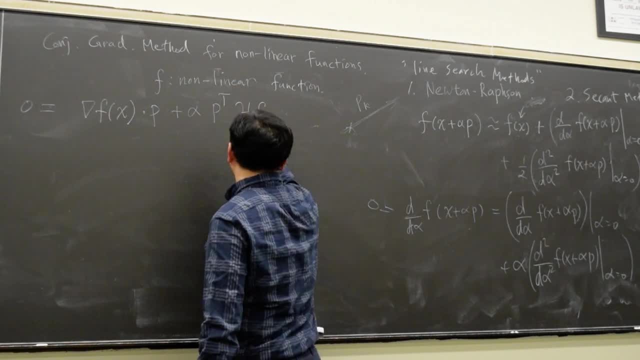 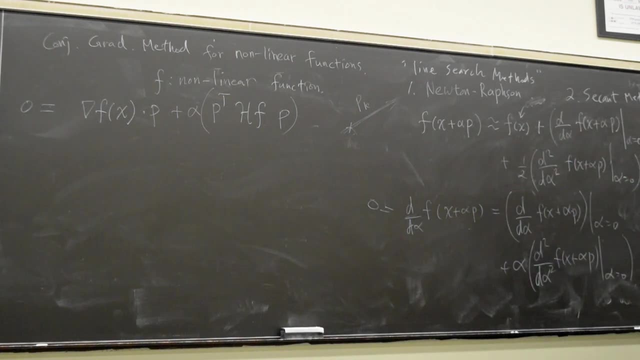 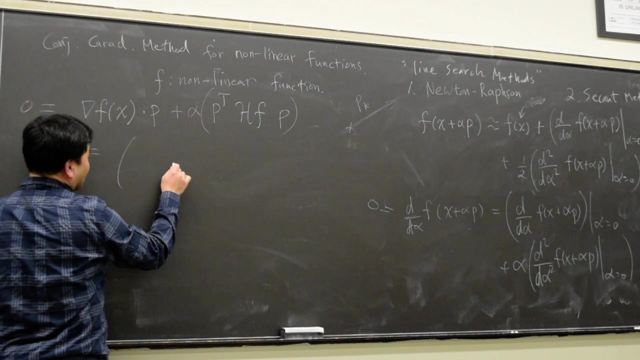 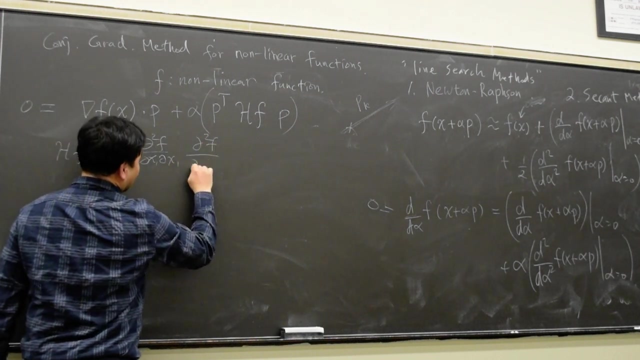 of f and you do p, transpose p, okay. So if you do that, then that's what you get, And your Hessian of f is actually just the matrix of second derivatives. It's just kind of so. it's a large matrix. 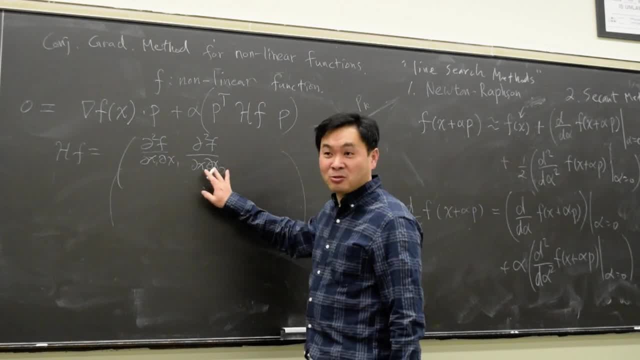 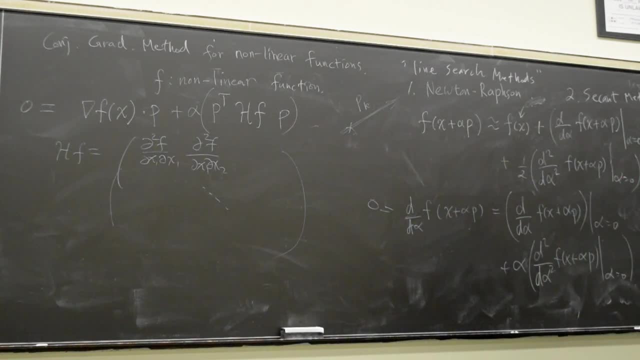 It does that, and it doesn't matter if you put x one first, x two first, It's the secondary, there's commute, so it's just a square matrix which is symmetric. okay, So you have this. Now we can even rewrite the dot product. 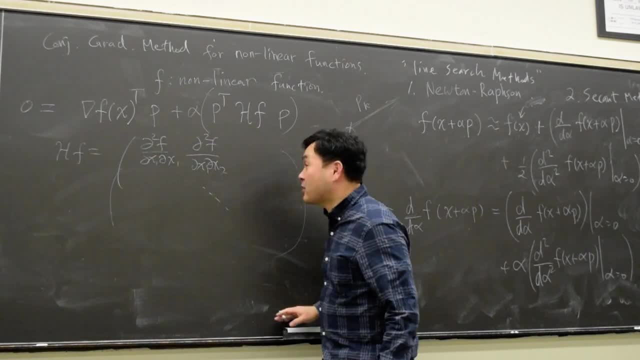 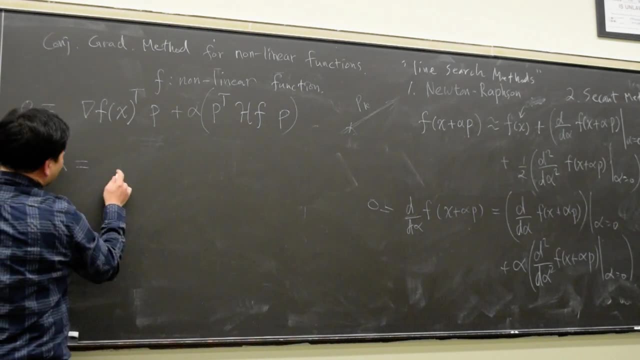 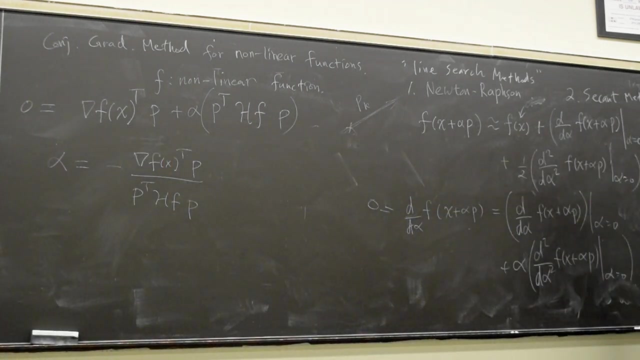 as transpose times. this because we're viewing these as column vectors And therefore, when you solve for alpha, we have alpha equal to negative gradient of f of x. transpose p over p, t, h, f, p. Okay Now. 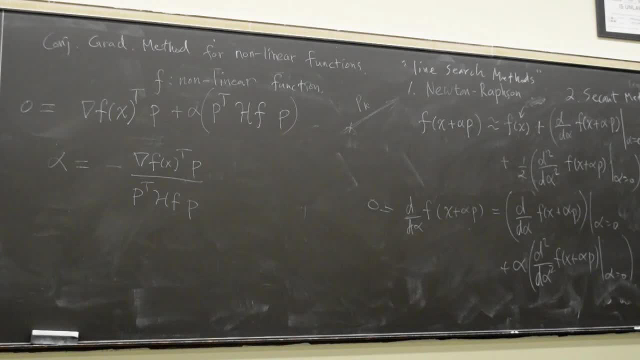 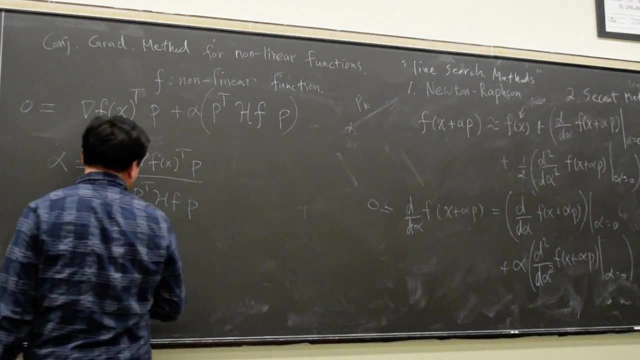 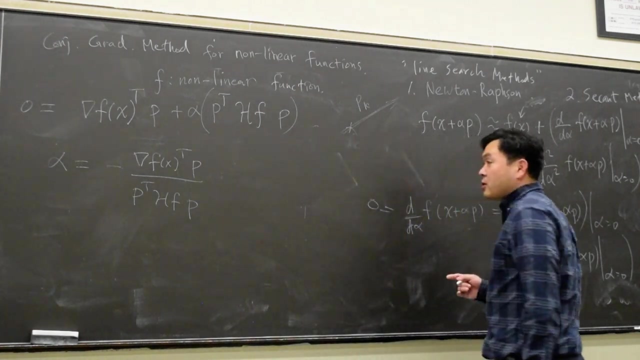 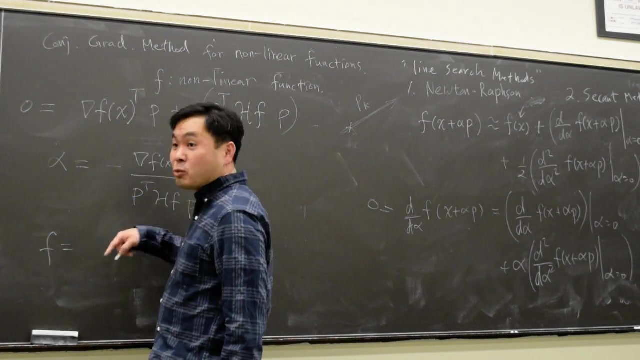 It's there, All right. Okay, let me cut it short, All right Now. at this point, I want you to think about what this means for the linear function, the quadratic functional, that we use for the regular, usual conjugate gradient method. 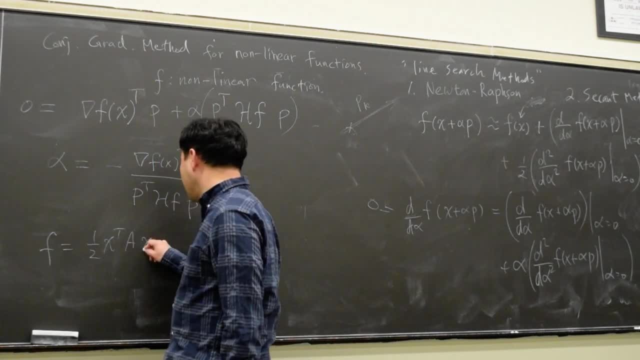 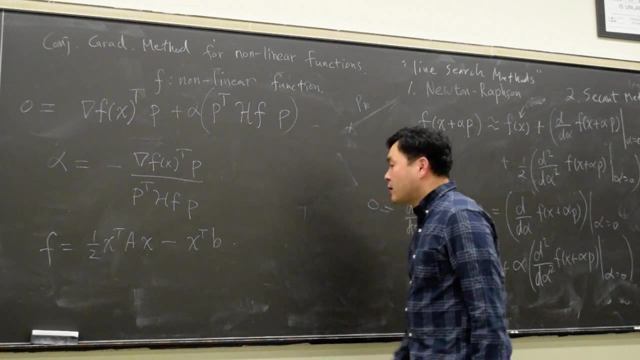 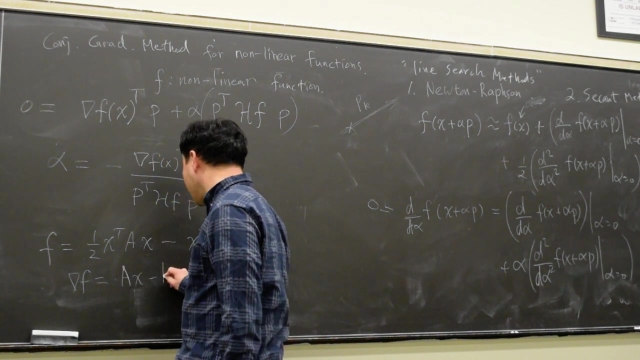 which was one half x t a x minus x t a. right Now, if you take the gradient, as I said, this is a x minus b, and if you take the derivative again, the Hessian is actually-. 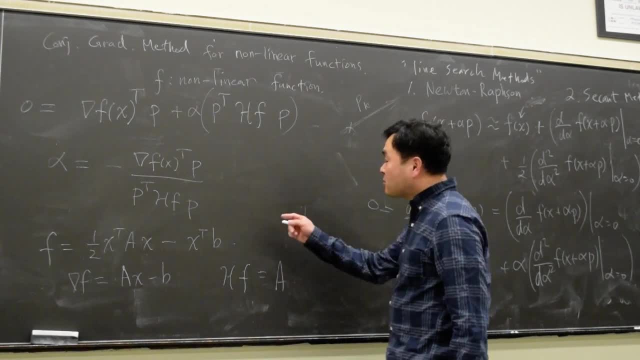 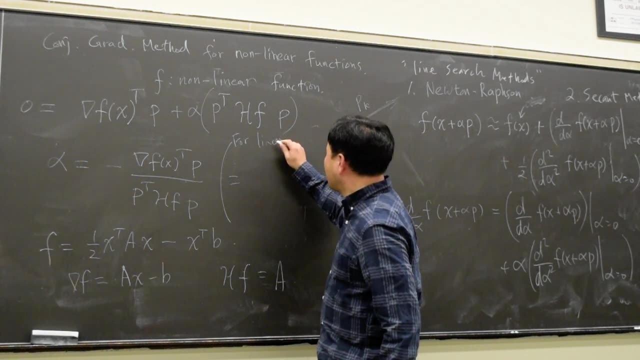 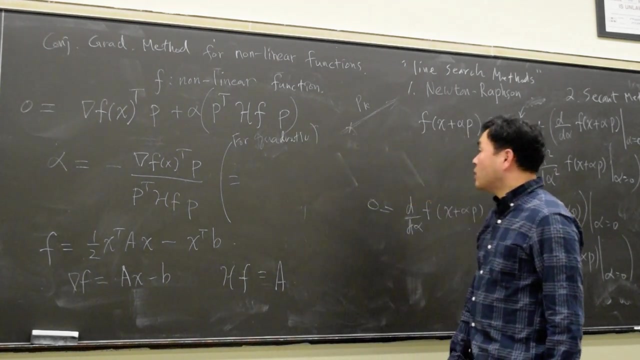 That's going to be a a itself. okay, So in the case for linear case, not the linear for quadratic case, This is a quadratic function For quadratic case. what you end up with is negative of this is your r. 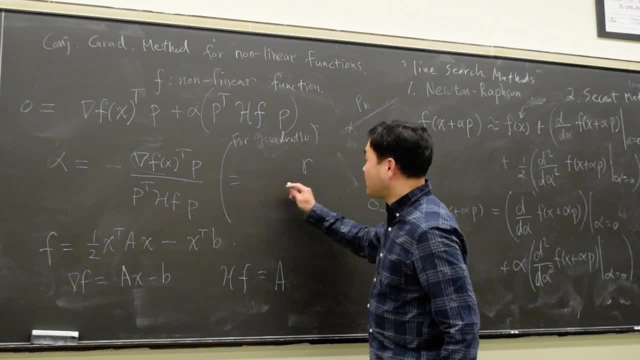 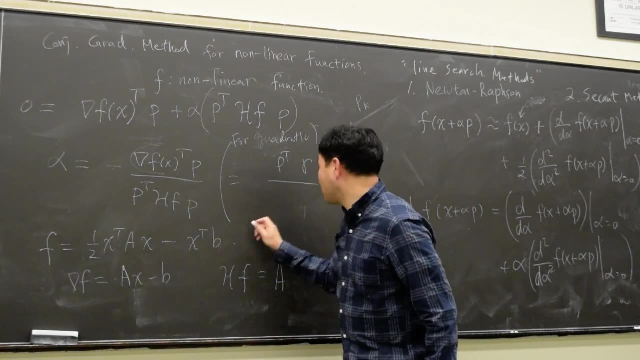 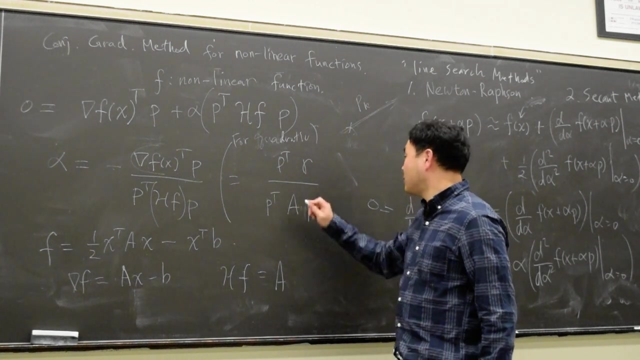 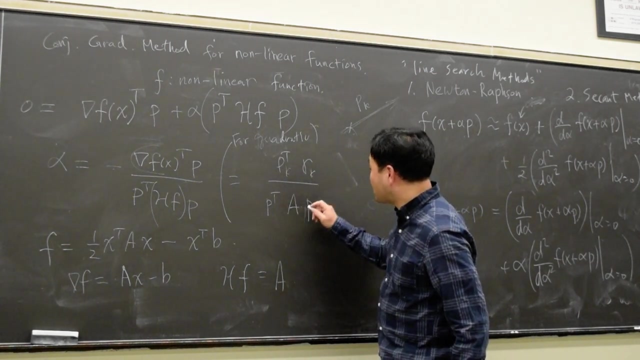 R, So that's really R, and then let's put PT here and then R here. So I switched the inner product And down here: this is your PT. A HF is A, so A and P, And we also in our previous presentation, we also figured out that this is same as RKT, RK. 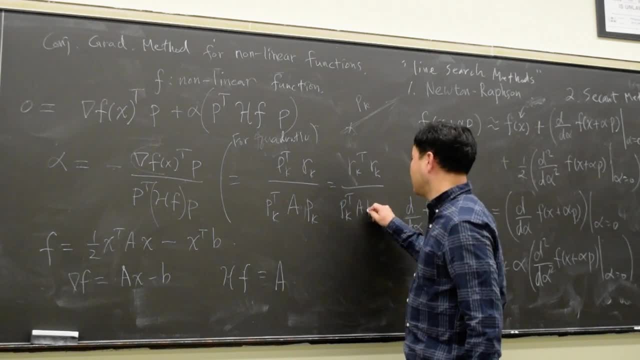 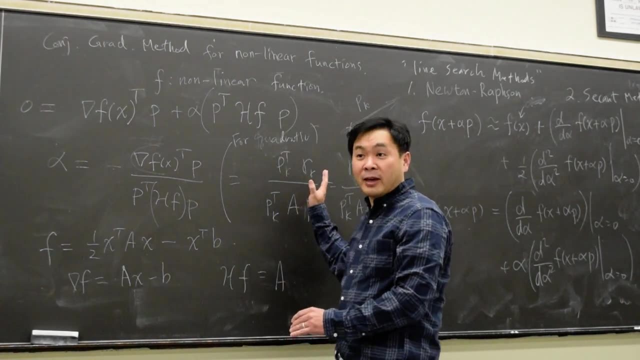 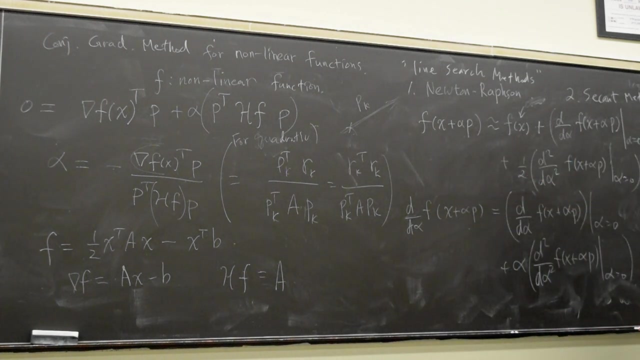 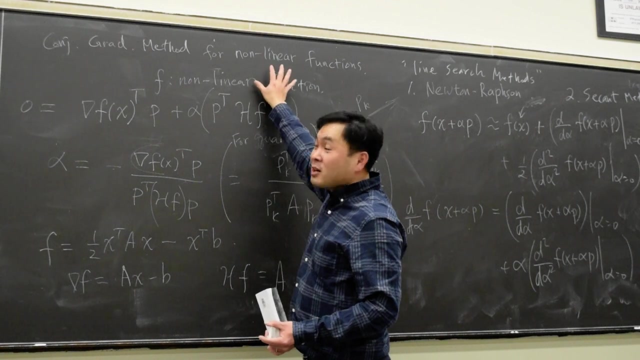 So it reduces to exactly the formula for alpha K when you have this one. So that's, I guess it kind of clarifies the relationship between this functional and general nonlinear function. What you're trying to do, What you're trying to do here is, if you're given a nonlinear function and you're near a minimum point, 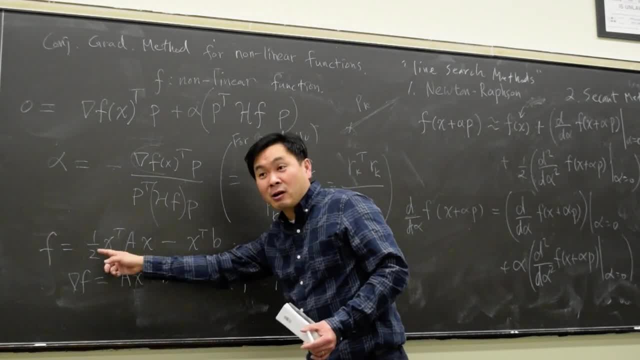 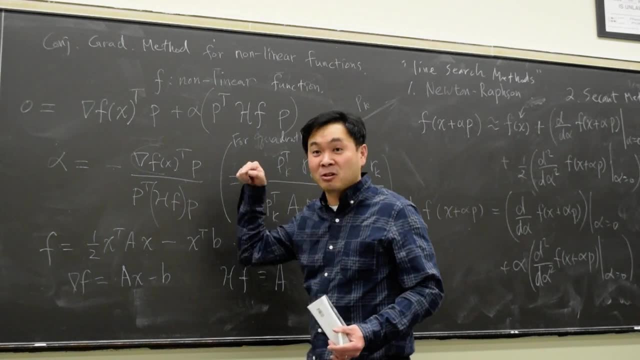 you're really thinking of it as some kind of a parabolic point, a parabolic function. You're approximating it as a parabolic function and you're trying to search the least direction by doing exactly that. So that's what conjugate gradient method does. 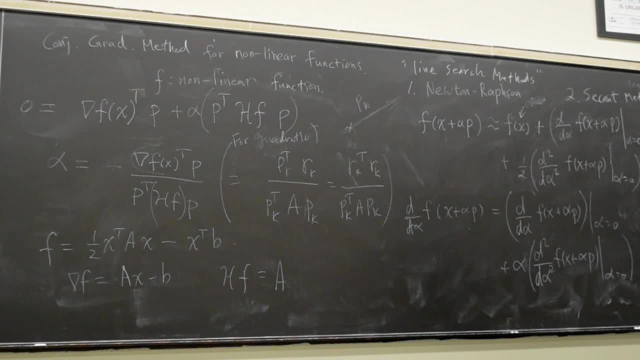 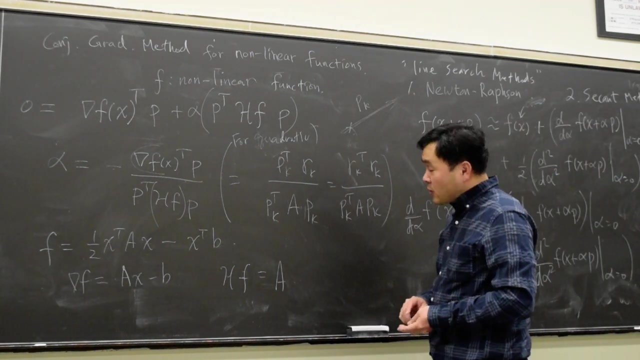 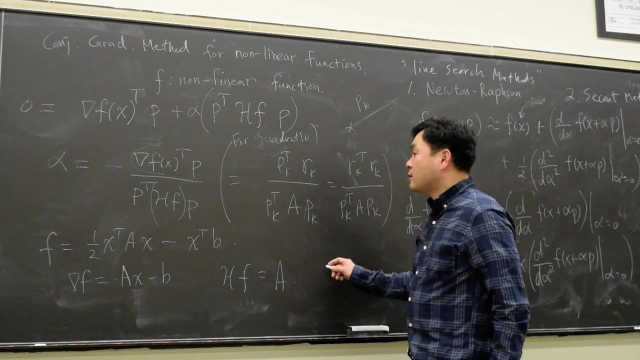 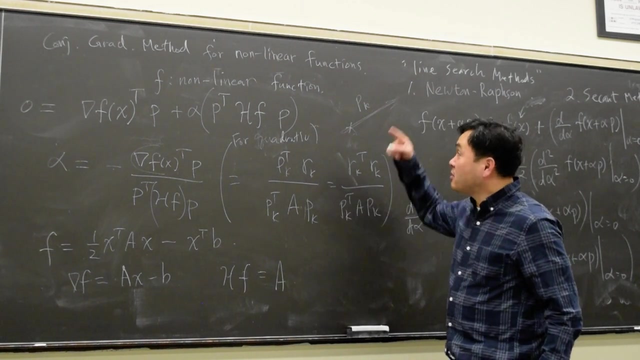 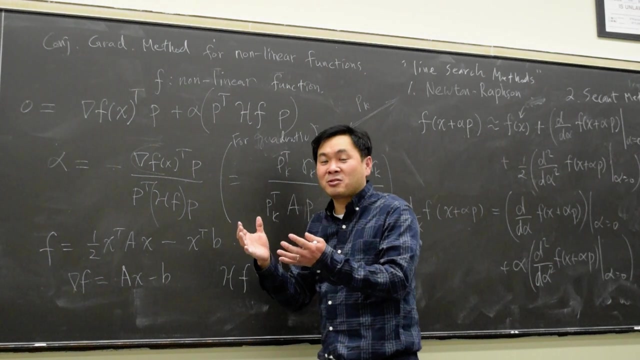 All right. Oh, and also another thing that you see is that, because this is the alpha K that you're modifying, and this entire system also will be very similar to the linear case when you're Near a. So you know, there's a mathematical theorem that says: if you have a minimum locally, 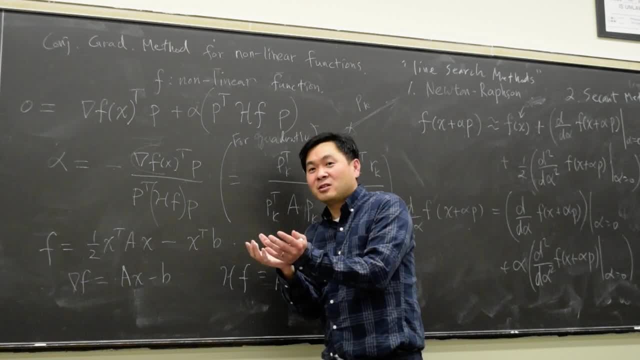 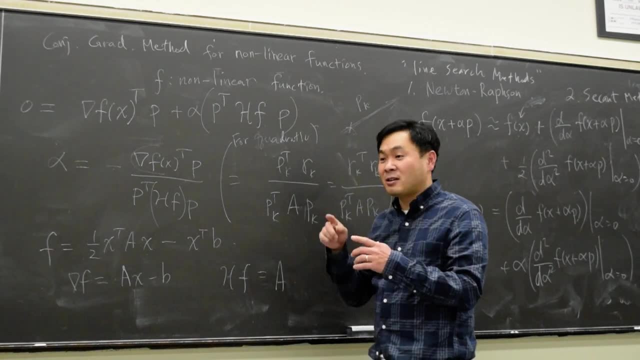 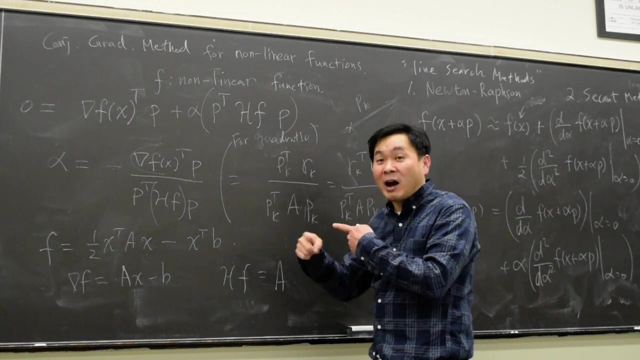 you can approximate it as a quadratic function, right? Yes, Yeah, So if you think about that, you can see that by looking at this relation, that near a singularity the PKs actually do become conjugate directions: Approximately, Not exactly, but approximately. 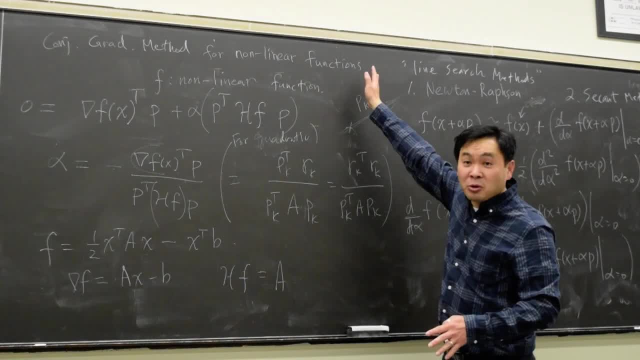 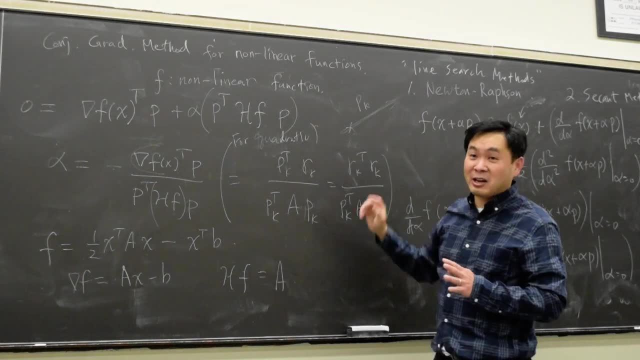 Okay, So that's why this method can still- It can still- be called the conjugate gradient method, although it doesn't make sense exactly. It's an almost conjugate gradient method, All right, So that's called the Newton-Raphson method using the Taylor series. 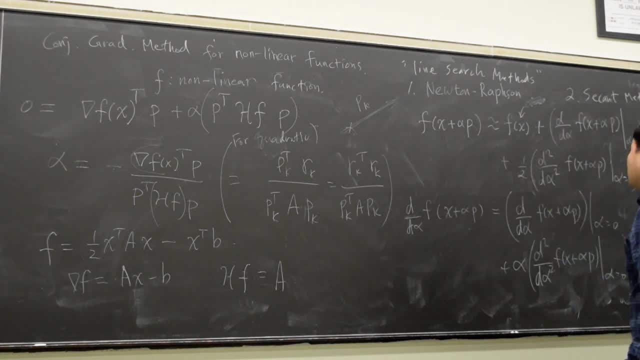 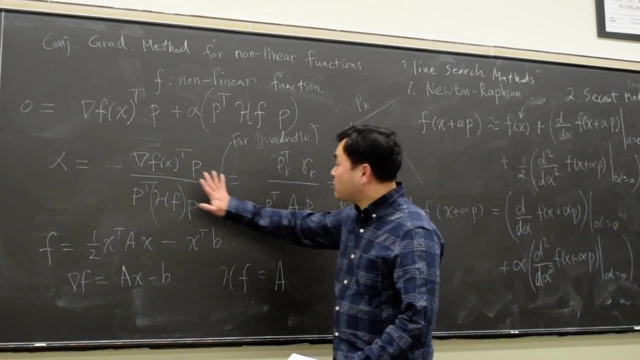 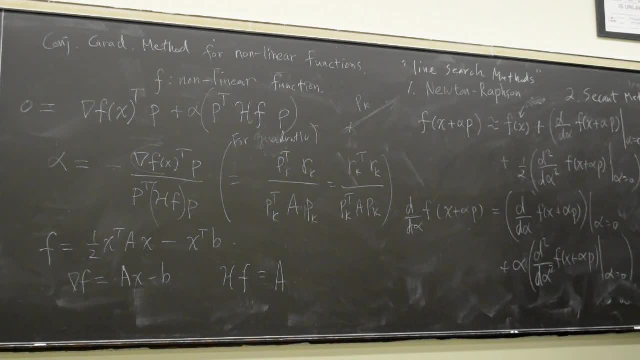 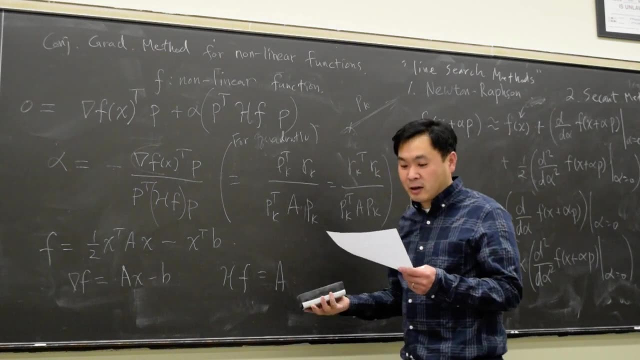 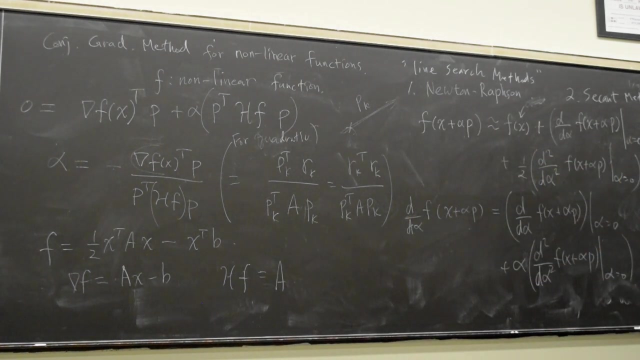 Mm-hmm And sometimes might be too much work. So you want to somehow approximate this H of F by using the finite difference. So that's the secant method. So if you think about where this came from, this was really here, right? 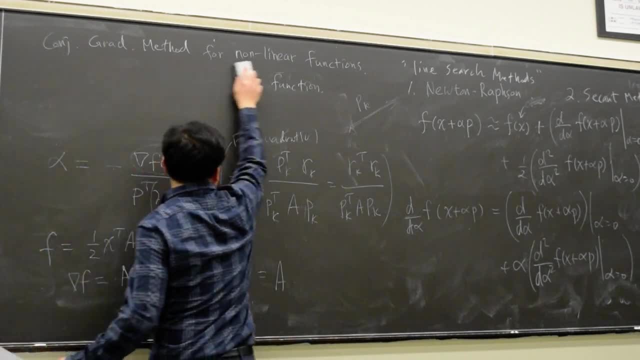 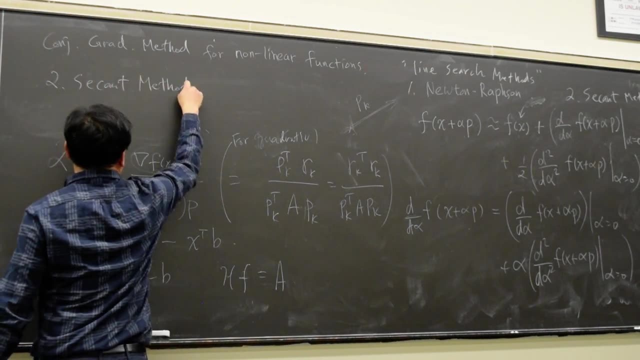 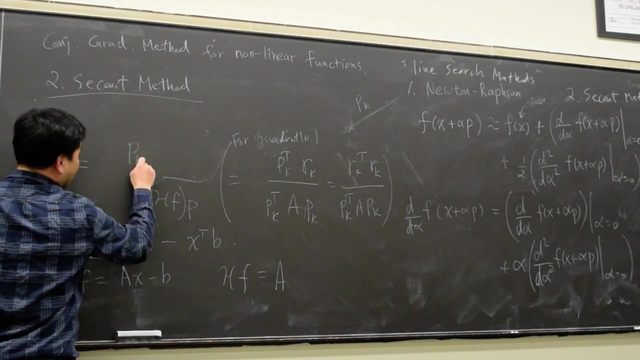 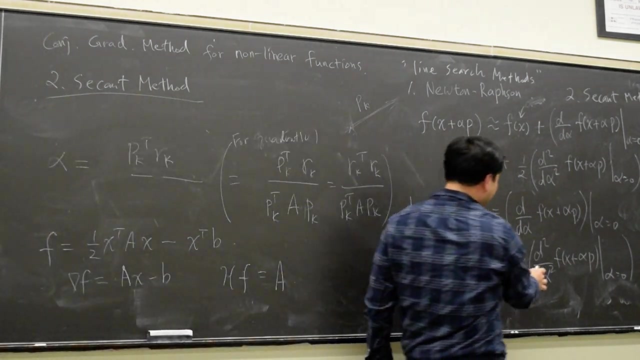 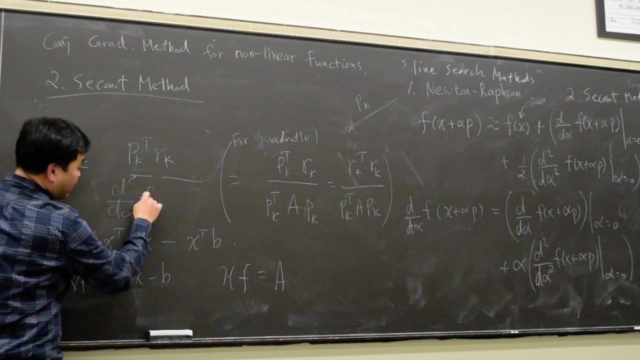 So if I do the number two secant method, then you're really doing the top will be the same as P, K, T, R, K, but the bottom one would be this thing here. so this would be D square, D square F of X plus alpha P. 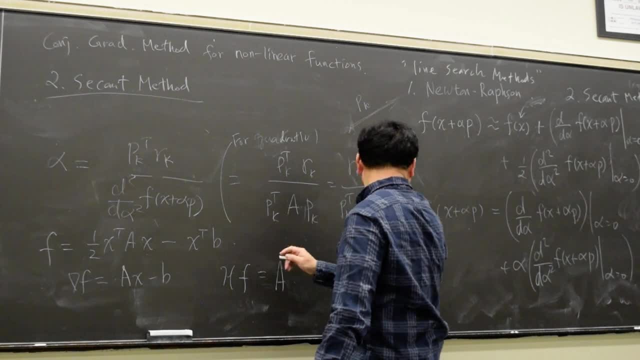 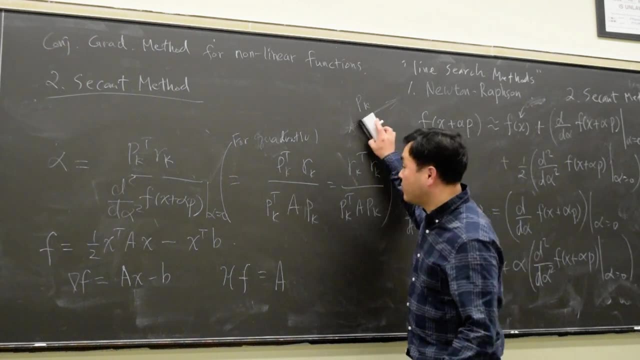 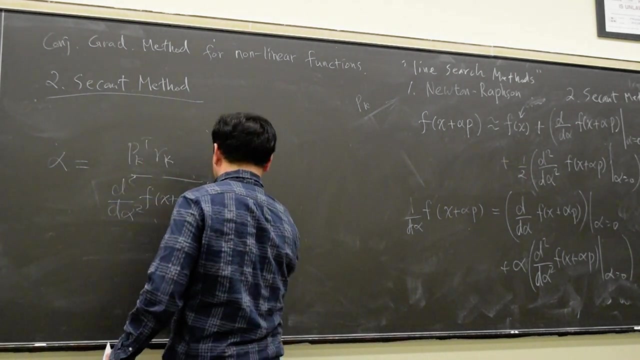 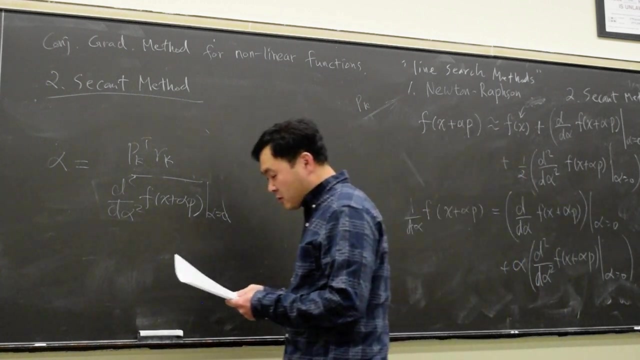 evaluated at alpha equal to zero. this entire thing is the same as P K, T, A P K. so let me erase this. so the secret method: we'll just say that this should be our choice of alpha K, except that we're going to say that D square. 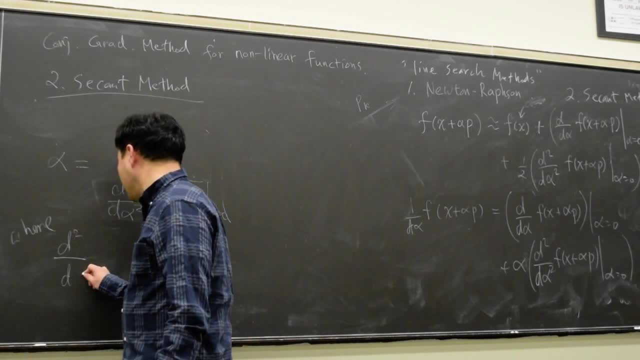 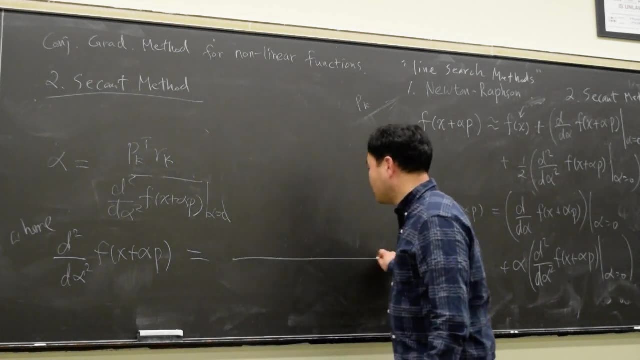 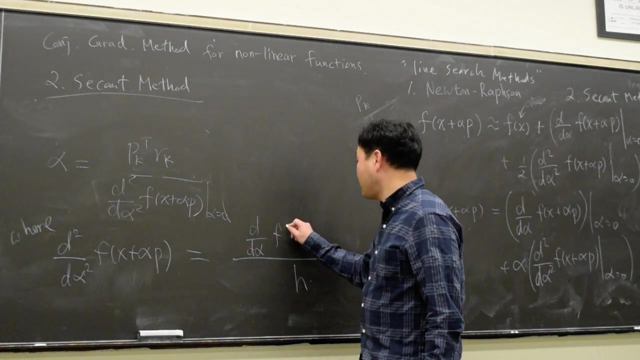 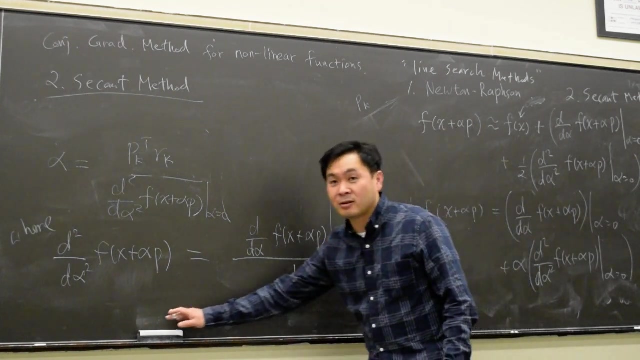 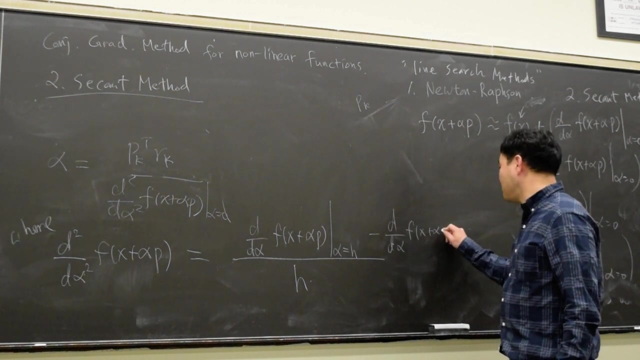 D D alpha. squared of F, X plus alpha P is equal to the usual finite difference H. and then you do D D alpha F of X plus alpha P at alpha equals to H minus D D alpha P, D D D alpha P, F of X plus alpha P.